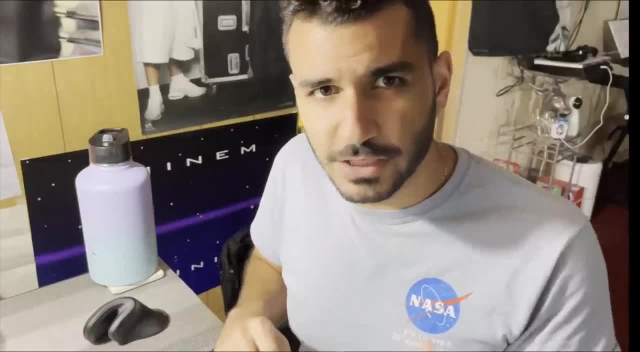 master's, and I'm about to finish up a PhD in electrical engineering. I've done many internships and research, so I'm really excited to walk you through all these classes, what I learned from them, which one was hard, which one was not, which ones were fun, and what to look out for. Let's just dive in. So as you can see over here, what I have is I have something called a flow sheet, and this 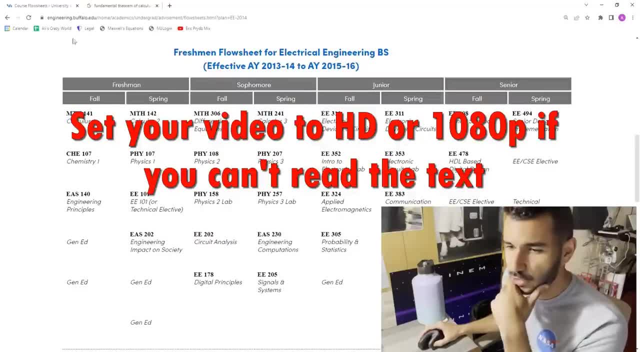 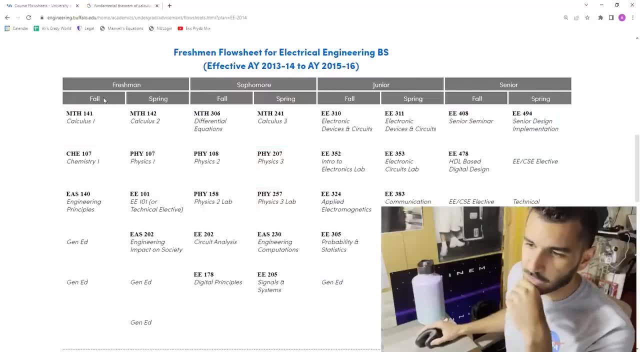 is something really nice that my university, the school I went to for my bachelor's, does is it lays out every single course from freshman, sophomore, junior, senior year, as well as defining it by your fall and spring, and this is basically the typical schedule you would take as an electrical engineering student, and what's really nice about this is if you were to like highlight a class, it shows you the prerequisites. So in yellow, we can see on the left over here, these two guys, like for example, in order to take that, you need to take calculus two and calculus one, but once you take calculus 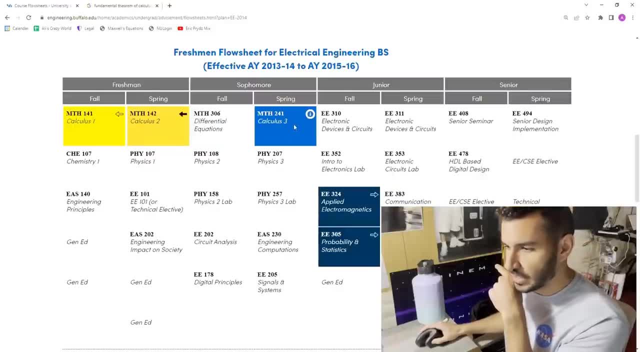 three, what that leads to is now you have the fundamental knowledge to learn, in this case, applied 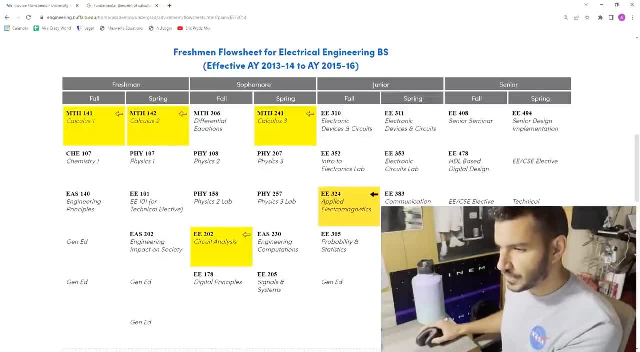 electromagnetics, probability and statistics, and energy systems. So I really like these flow sheets 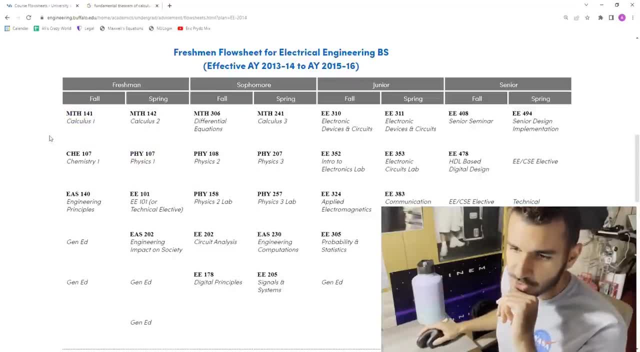 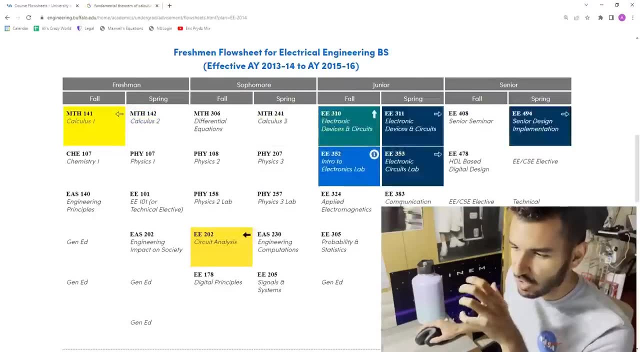 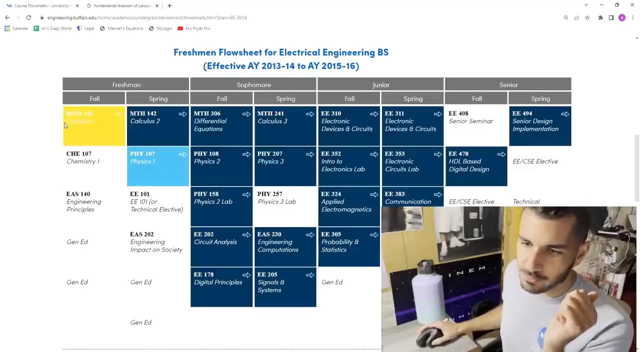 because they really give you a quick understanding of what's going on. So as far as your freshman year, I'm going to go through the freshman year classes pretty quickly because I basically want to get into the meat, the hardcore electrical engineering classes, which is sophomore, junior, senior year. So freshman year, you basically take calc one, which is basically the branch of 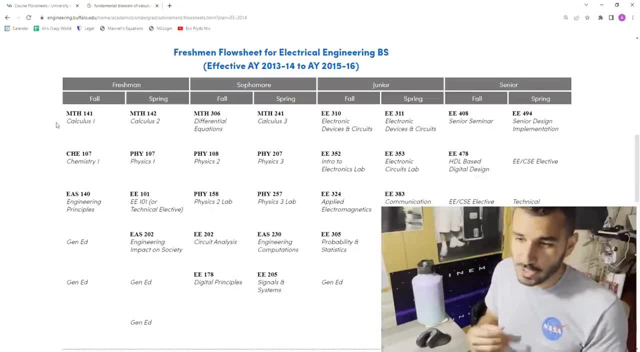 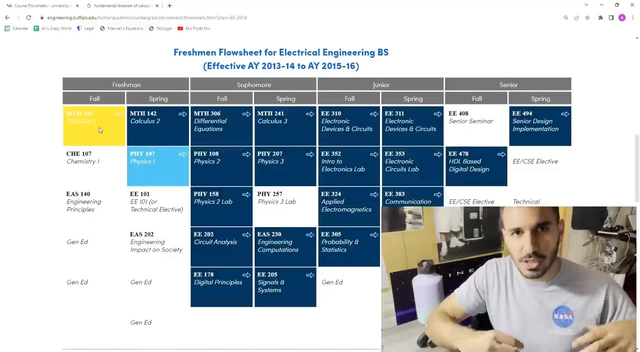 mathematics that deals with rates of change, things that change, and basically being able to measure how fast they change or how slow they change, and that's pretty much like the fundamental idea. You learn about the fundamental theory of calculus, and you basically take that as, and obviously because in the real world, things are constantly changing, and when you're doing physics calculations, 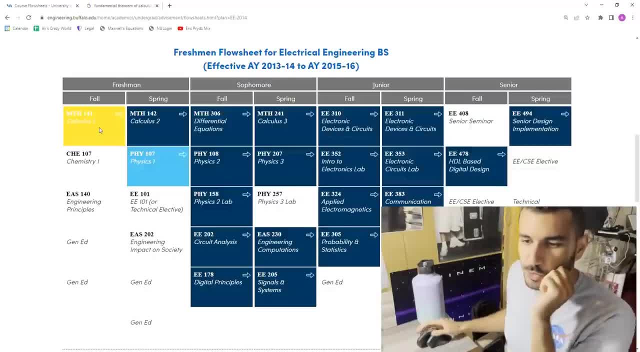 you want to understand how fast these things are changing. Calculus is extremely important. Now, I want to talk about chemistry one, which I don't really understand why chemistry is taught for 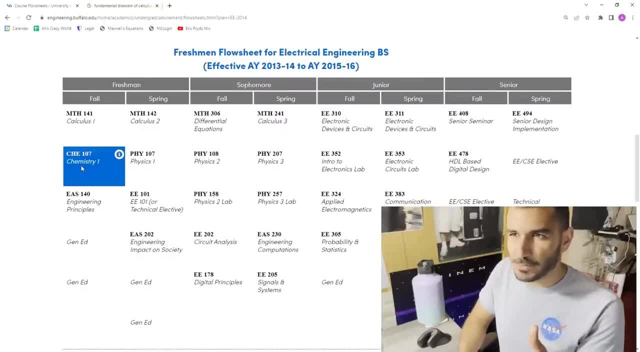 electrical engineers. The only thing that would make sense is because in the first chapter or one of the first few chapters, you learn about charges and molecules and atoms, which really these things are branch of physics, but they're kind of grouped under chemistry. So that is kind of relevant when you learn electromagnetic physics. However, some of the stuff later down the line, like the reactions, 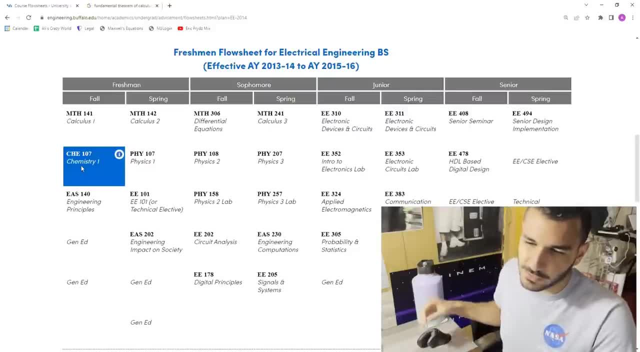 whatnot, I really don't think it is quite useful. However, it is, I guess, freshman year class. So it was okay. 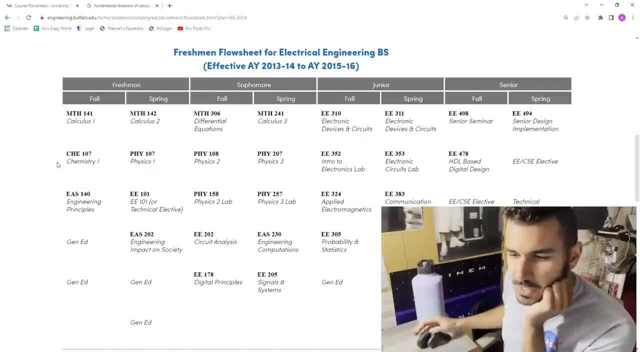 I think I got an A minus in this class. I wasn't really a big fan, but it was okay. Then there's this engineering principles class. And I think in this class, what you're supposed to do is like 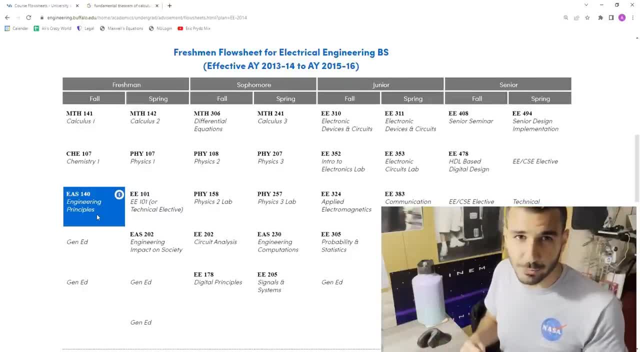 build a wind turbine. I didn't take this class. Instead, I took an introduction to computer science 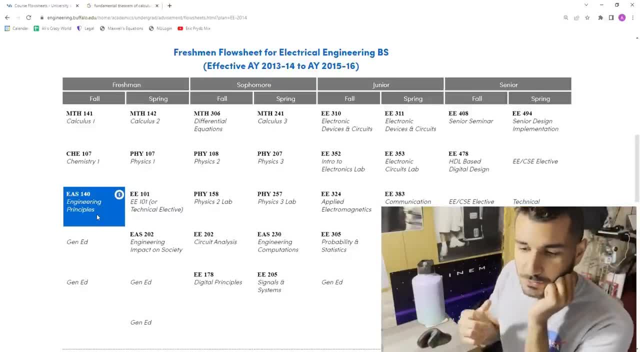 because at the time I was still debating about computer science. And even though I did like the computer science class, that was, I didn't end up going with computer science and I have a separate 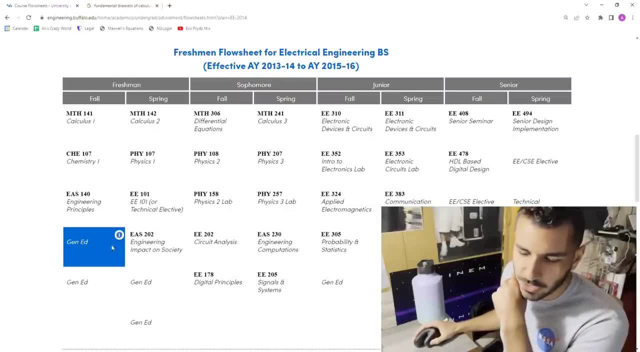 video about that. I'll put it in the description. And then for my gen eds, I took a writing class, 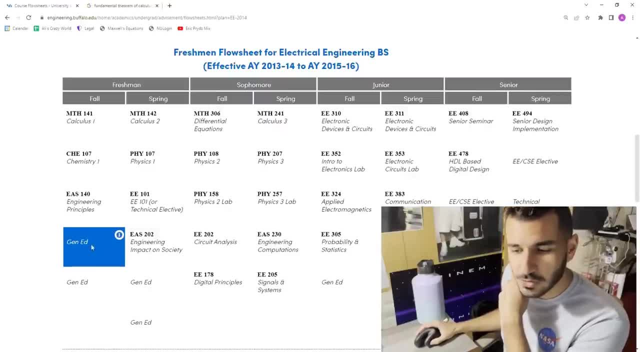 and then I took something else. I forgot like some type of seminar and writing was really good. I ended up being a really good teacher. So that was good. In the spring, I took calculus two, which is a 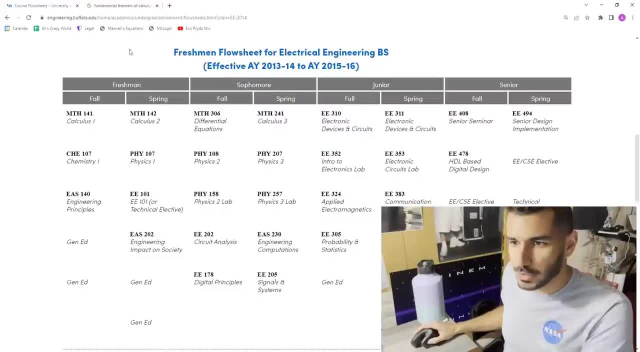 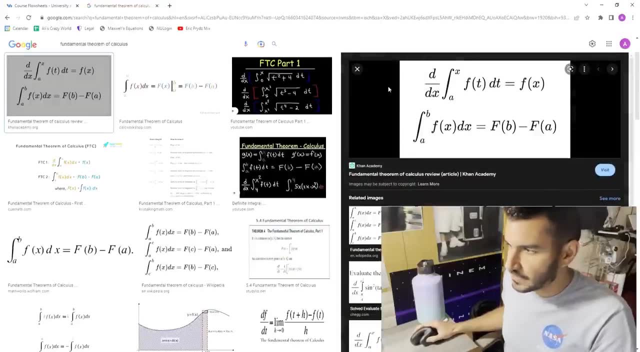 continuation of calculus one and where calculus one deals with differentiation. So which like basically stuff that looks like this derivatives, like you see D over DX, you take a variable and you're calculating how much it changes with respect to some other variable. Very often time 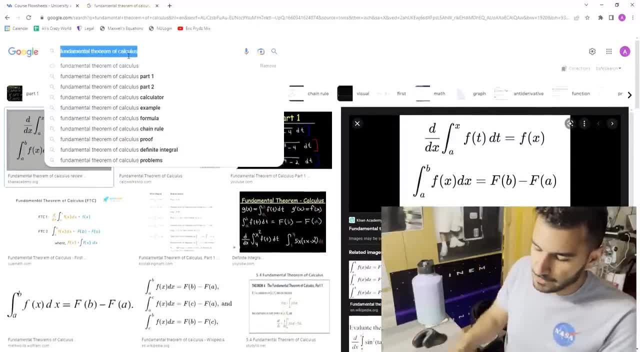 would be the thing that we write derivatives off of. There's in calculus two, we learn about integrals and you're just kind of like doing the reverse where you're taking, 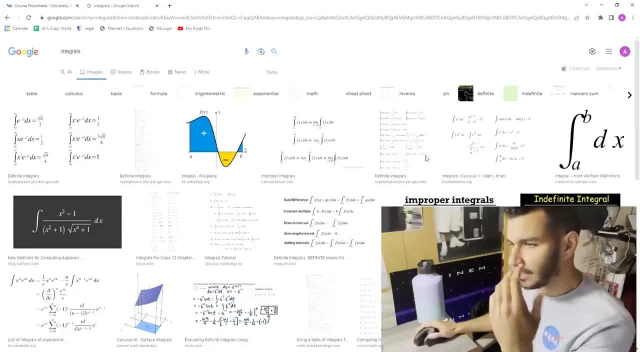 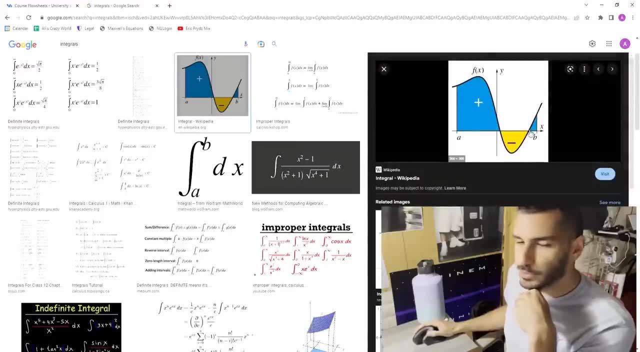 um, a bunch of little things, adding, adding them up. And an integral really is just the summation of, of something. So for example, if there was an F of X, this black line, uh, the derivative will show you how, how this black line is changing. Uh, the integral will basically show you the surface 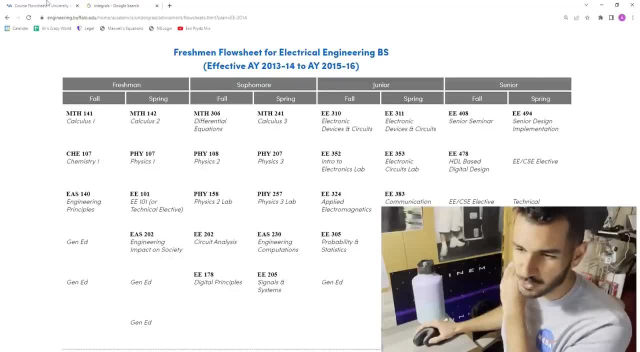 area under the curve. And if all of this is flowing over your head, don't worry. Once you take calculus two, uh, you'll get to have fun with that. But basically again, it's just continuation 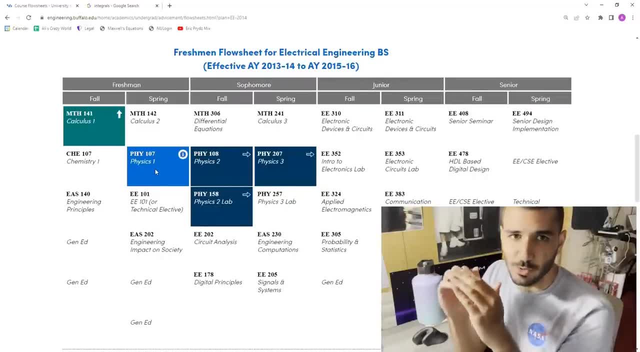 of that. And here you take physics one and physics one deals with mechanics. So basically things that are macro and like things that move motion forces like a rocket launching 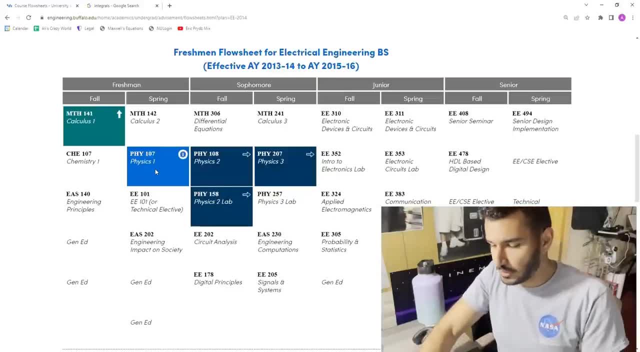 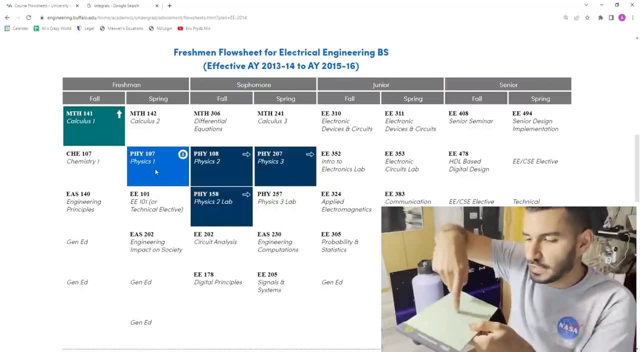 into space, like a ball falling, uh, like a friction. So if I'm, if I'm, if I'm rubbing my hand across this paper, like how much force do I need to keep it going? And how much friction is the paper, uh, creating and force and whatnot. So this class is really the basics of like 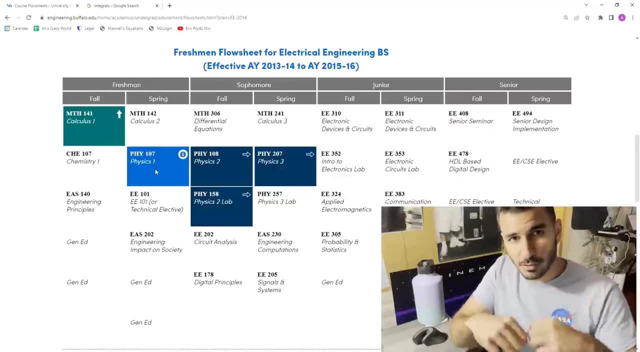 mechanical engineering and civil engineering and all the types of engineering that deal with large things. Of course, we electrical engineers deal with small things on the microscopic level charges and fields and waves. Uh, so that's where physics two comes in. 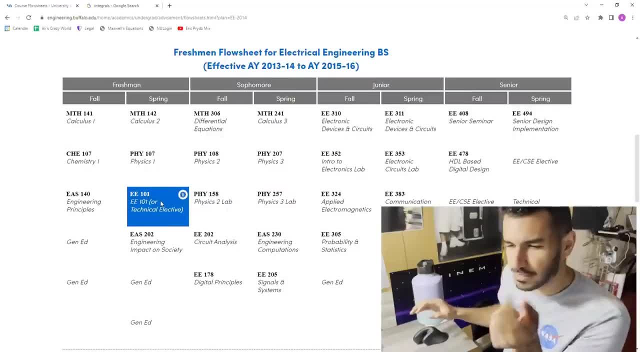 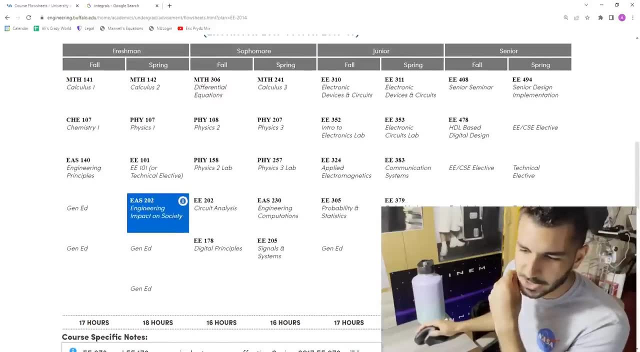 Now there's this EE101. Um, I think this was added after I graduated. I don't really know what this is. I'm guessing some type of class that teaches you like some introduction concepts, uh, engineering impact on society. I didn't take this one, but I think this class was like just people presenting what it's like to be an engineering. Instead of doing that, I would basically go and talk to 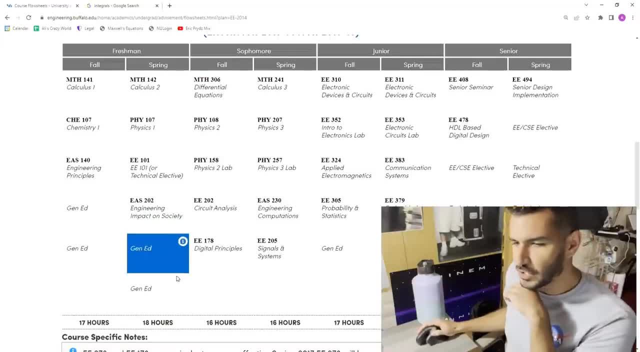 engineers in the real world. And I'll talk about that towards the end of the video. And then for my gen eds, I think I took rock and roll engineering. And then I took physics two. And then I took 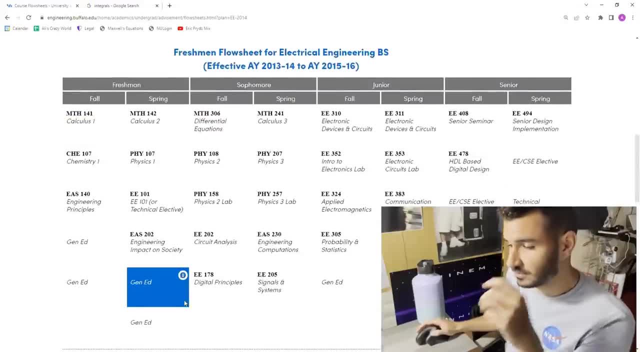 history, which was awesome. That's probably one of my favorite classes where I met one of my friends who ended up being, um, one of my study buddies and then sophomore year. So that takes care of 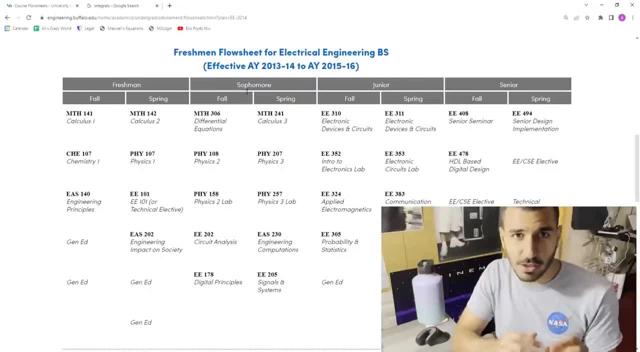 freshman year, sophomore year. Okay. You have a good understanding of the math and the physics involved. And then you're basically getting better at the math and physics, the skills that you would need, but you also start learning some electrical engineering concepts. So differential equations is basically a continuation of calculus. It's branch of math that deals with, um, like 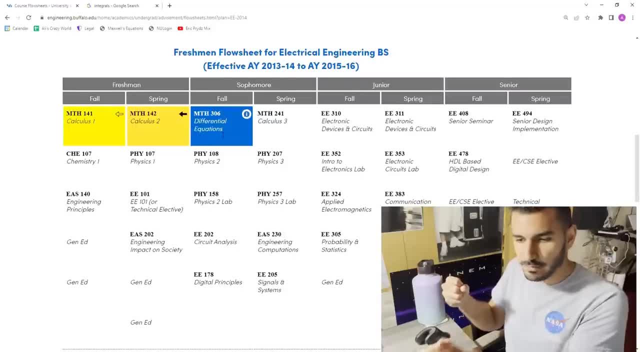 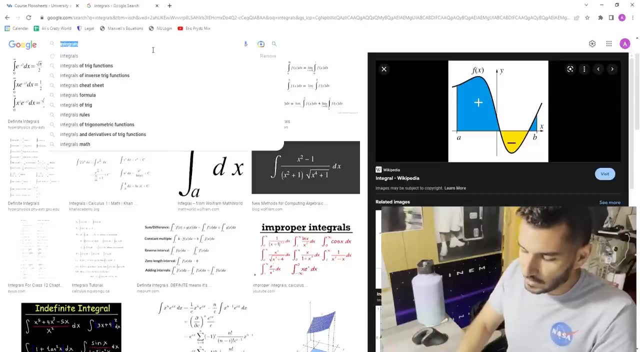 so, so you take, so, so you take a derivative and, and, and one variable within the equation, but then other variables are not necessarily changing. And what I mean by that, for example, if you go and learn about, uh, like capacitors and inductors, um, so capacitor differential equation, for example, 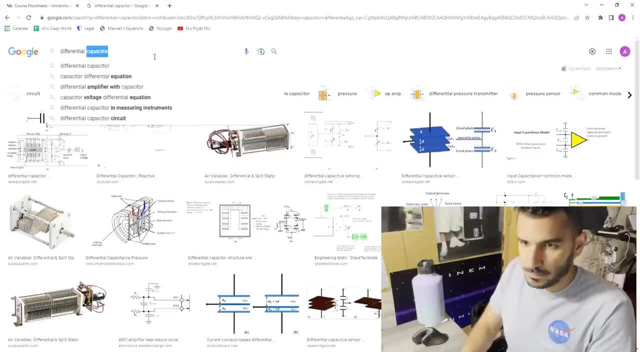 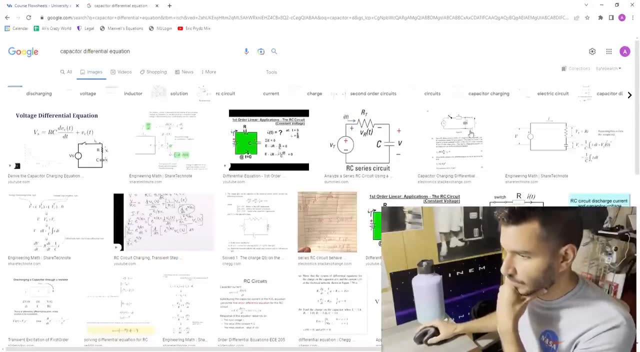 capacitor differential equation, you'll see in the equation of capacitors, for example, let's look for a differential one, right? 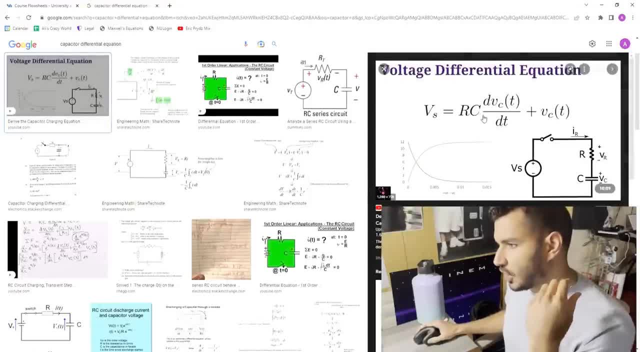 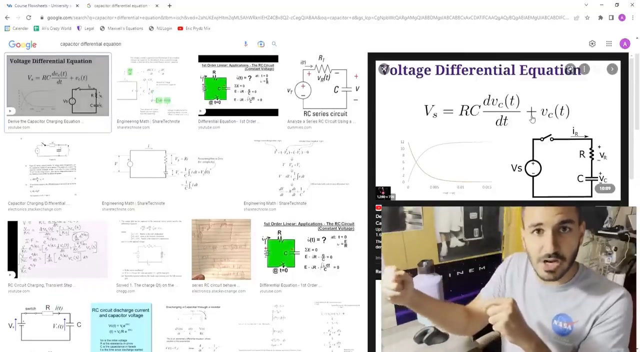 Here. So in this case, you have a voltage, you have resistance, you have charge, or I'm sorry, it's capacitance, which depends on charge. And then you have suddenly, so you have these, these variables, um, and then you have a derivative, you have a DV over DT thrown within that equation plus, uh, like a VC in this case. So this is a differential equation because one variable is changing while another variable is constant, for example, and we basically learn about that. Um, and again, once you get into it, 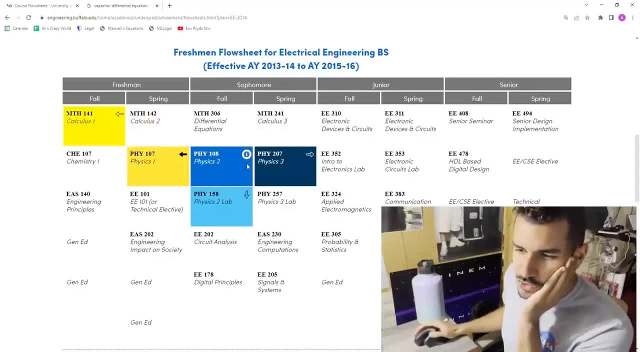 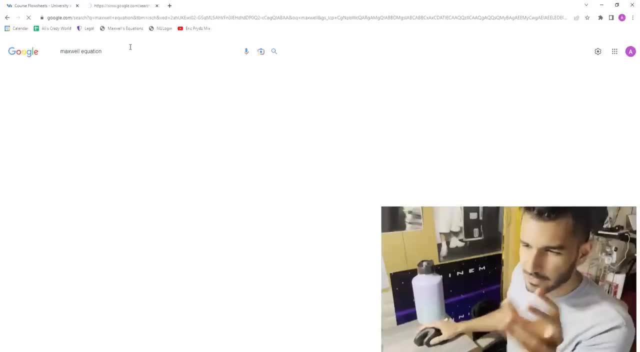 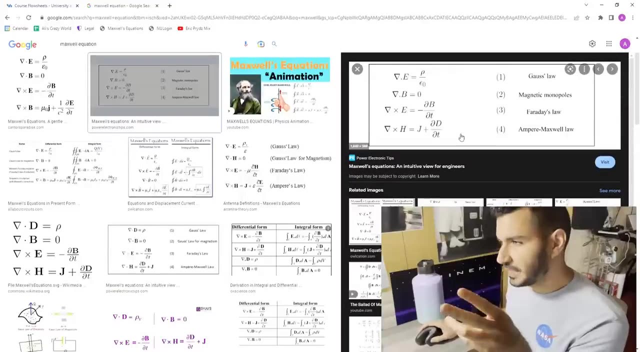 that's basically the gist of it, you do a lot of exercises. Physics two deals with electromagnetic physics. So that's where you start learning about electric fields and magnetic fields and Maxwell equations. You get like a very basic introduction to these four guys. And I know these kind of look either really weird or simple or really complicated, but they really just pretty straightforward. First one tells you that an electric field exists because of an electric charge. Magnetic field does not exist on its own because there's no such thing as a magnetic charge. 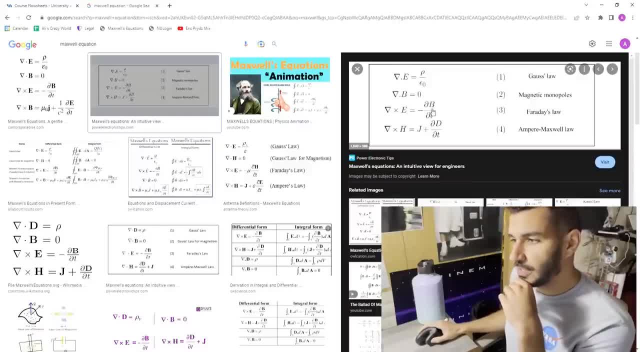 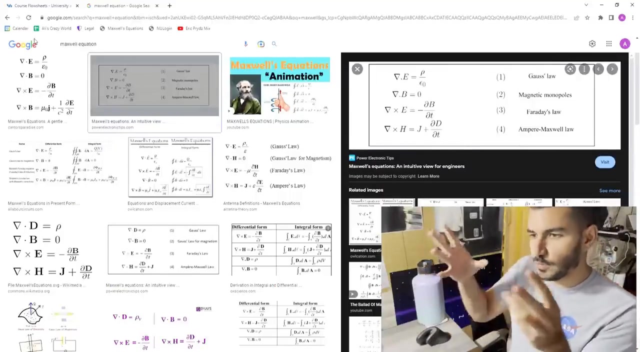 Third one says that. That a changing magnetic field. So right here, there's a derivative that we see the rate of change of the magnetic field with respect to time will induce an electric field. And likewise here, if you have a charge, you'll have a changing magnetic field. If you have a charge, uh, you'll have a changing magnetic field. And if you have a changing electric field, uh, you'll have a changing magnetic field as well. And this is basically the four equations that define the behavior of 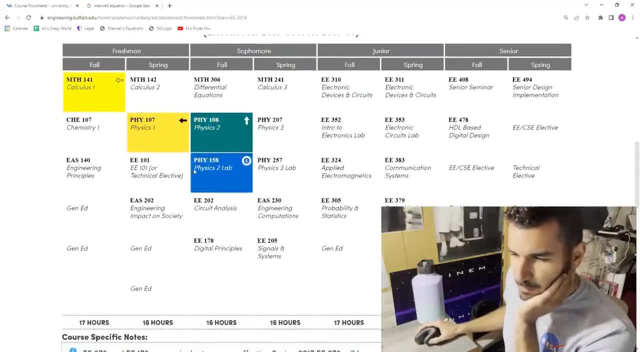 electromagnetics. Um, and that's basically where you learn that there is a lab component. Which is kind of, it was okay that the labs themselves were fun. The write up was kind of boring. Uh, you have to like write an introduction. No, that's okay. Circuit analysis is a very 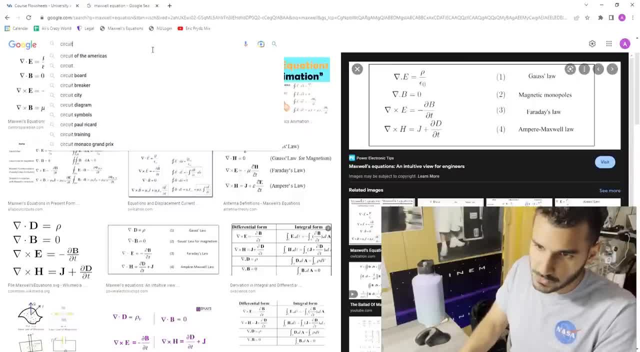 important class. It's the class where you learn about circuits. So circuits, uh, circuit analysis. 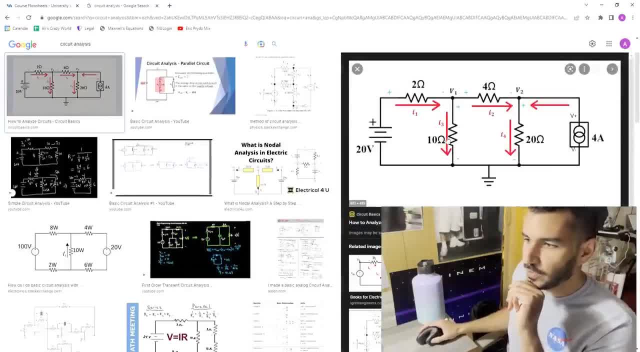 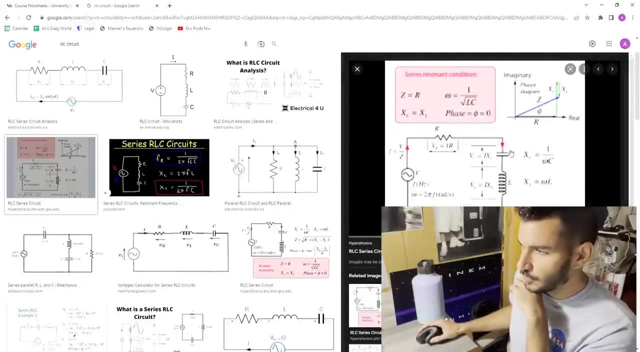 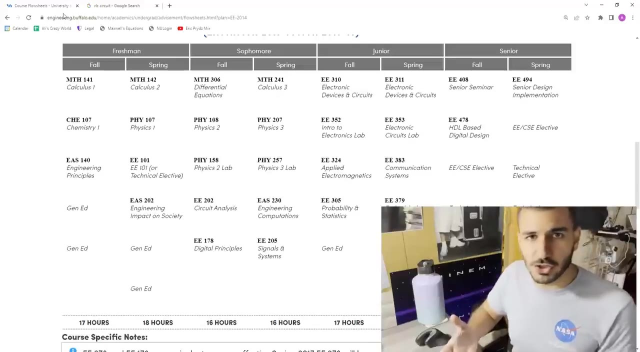 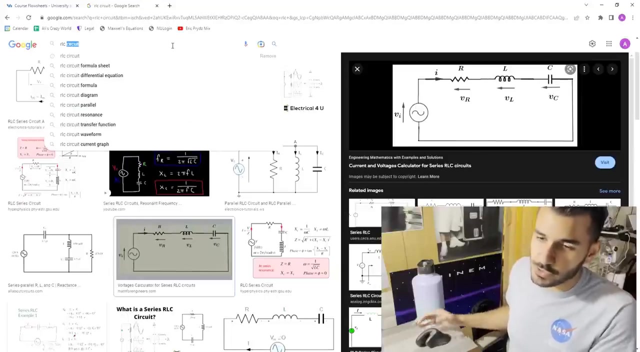 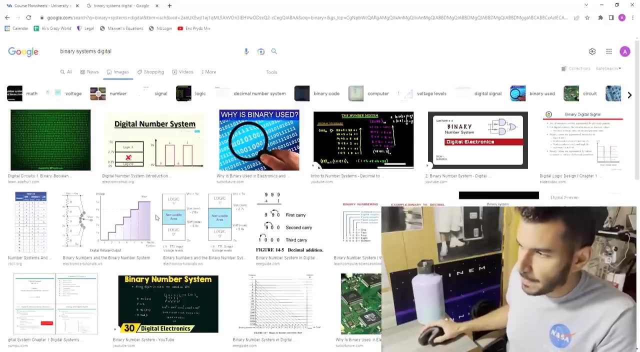 So you basically learn the basics of how to solve circuits. So basically what is a power source? What is a resistor? What is amperage? And you basically do that. And then later on you introduce capacitors and inductors. So there's RLC. There's like later on in the course circuits that look like this, you introduce other components, capacitors, inductors, and you maintain this voltage source. And this is actually a really good class because this class is the foundation of electronics. Um, so if you're interested in electronics or like how all the circuits around you work, this gives you a very fundamental understanding. And then finally there's digital principles, which is a class that deals with ones and zeros and how to use them to build things in the real world. So like if we look at binary or binary digital systems, um, like just basically ones and zeros, we take those. 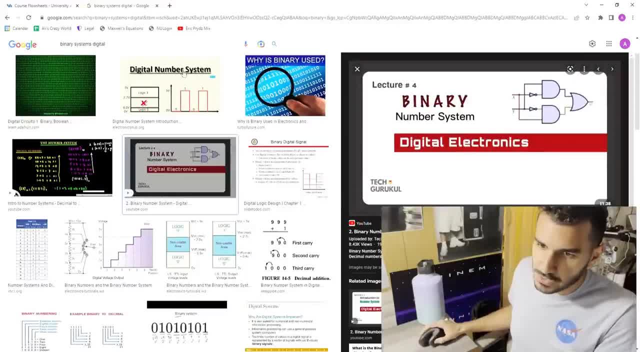 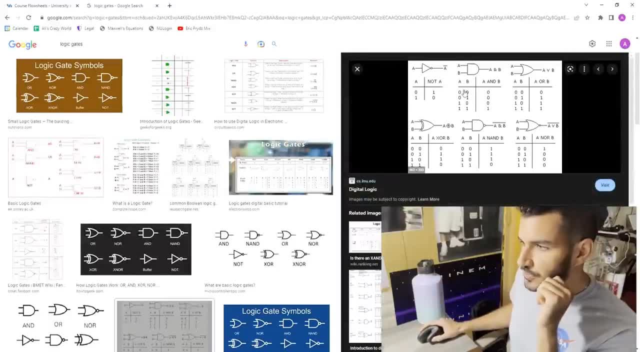 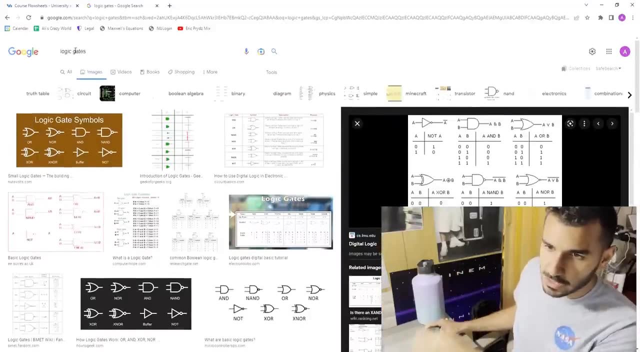 And then we built something called logic gates that look like this. So logic gates are basically the foundation, the building blocks of taking like ones and zeros and being able to do mathematical operations with them. And then we basically use trends. We use circuits, we use transistors to build these logic gates. So if you look at logic gate transistors, 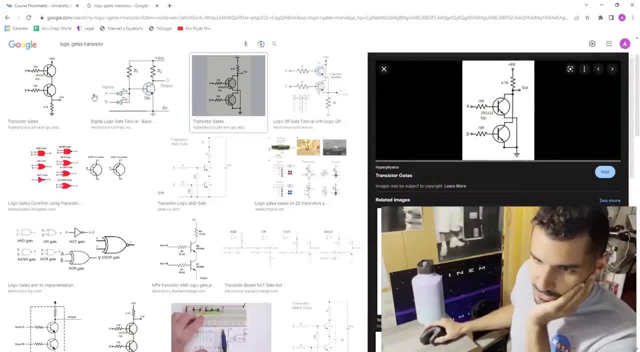 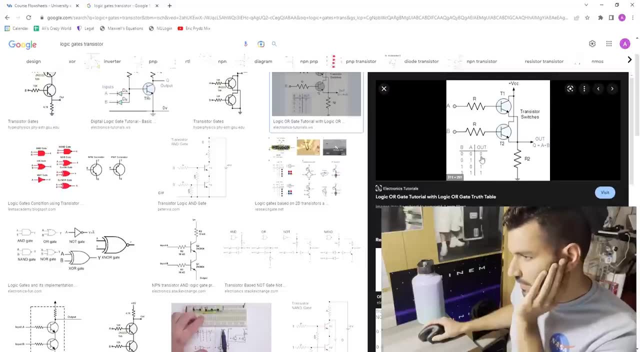 um, this is essentially what it would look like. Like this is one type of logic gate other. Um, there are some diagrams that in this case, this shows you. So in this case, um, this is like an and there's an and gate, and this is how you would build it. And this is 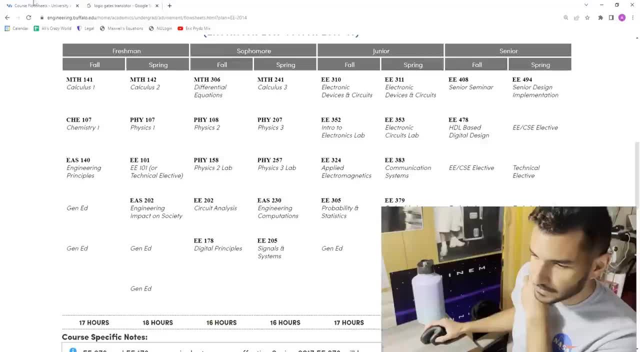 the foundation of modern computer engineering. So if you really like this class, digital principles, like you really, really like it, you're absolutely fascinated by it. You should consider looking into 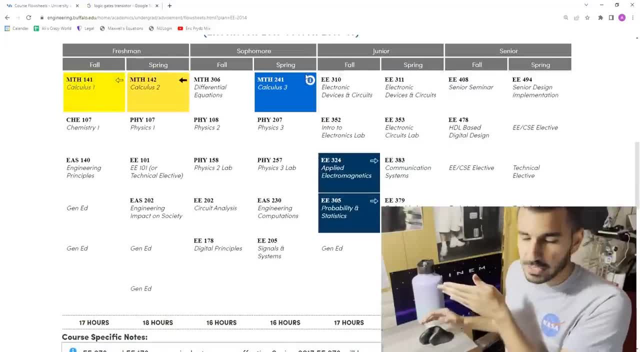 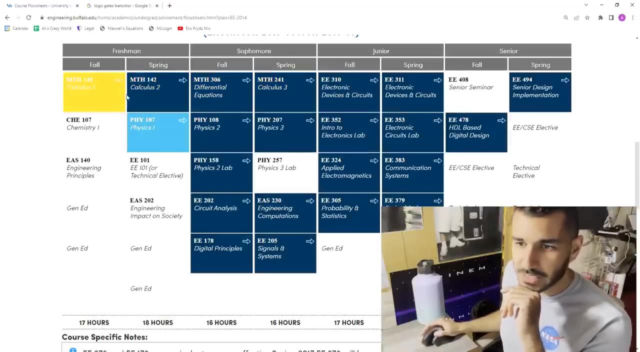 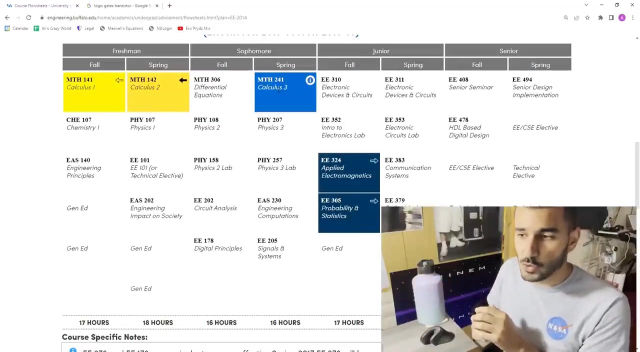 computer engineering as a major. Um, and the spring you take calculus three, which is a continuation of Calc one and two, although more Calc one, because it's really fo still focusing on differentials and integrals, but now it's applied to multiple variables. So in Calc one and Calc two, you do derivatives and integrals only with one variable, but in Calc three, you start doing it with multiple variables. And this is, this becomes very relevant to electromagnetic physics because electric electric fields, for example, they flow in three dimensional, um, 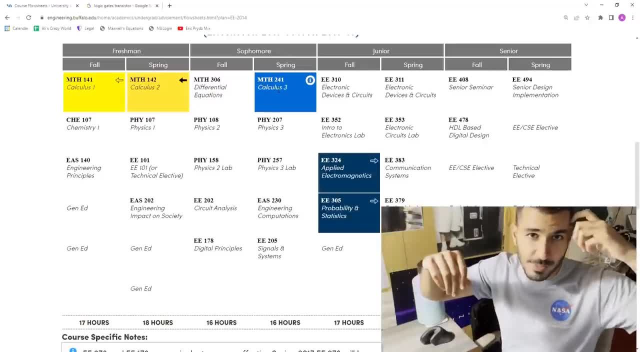 space or like a gravitational field flows in three dimensional state space. So now you have to define X, Y, and Z, and not just X or not just time. Um, so that's basically what you're doing. 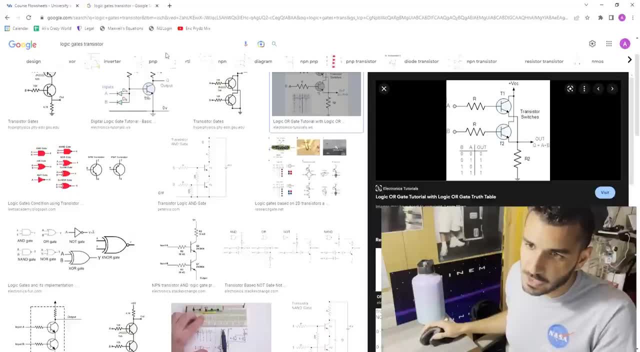 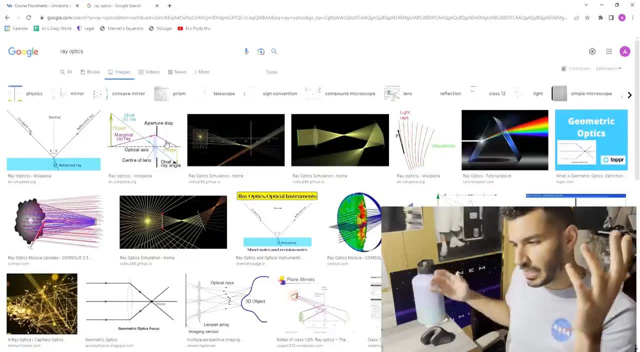 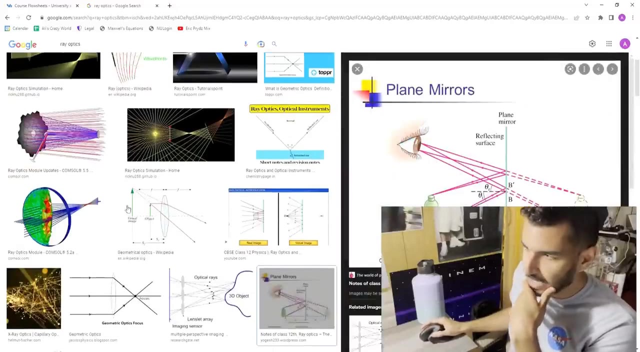 In physics three, you learn about optics and waves and mostly optics, like ray optics, and it would look something like this. So you, you basically learn about refraction, reflection, diffraction. If you don't know what these things mean, that's okay. That's essentially, uh, what type of behavior waves will do and lenses and how do lenses behave and defining lenses and focal 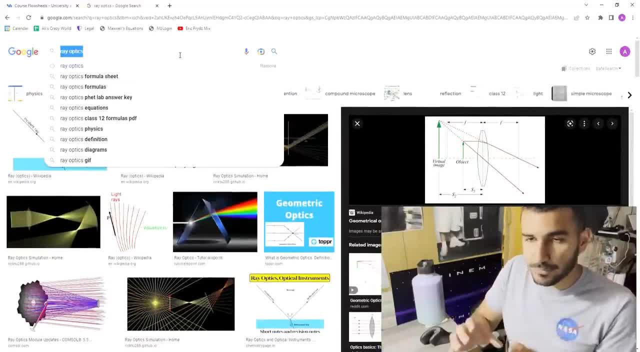 points. Uh, that's really the core of it. And you also learn about very important fundamental diffraction concept, which is the single slit experiment. 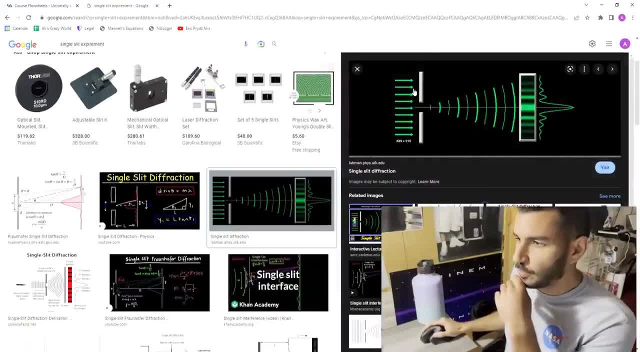 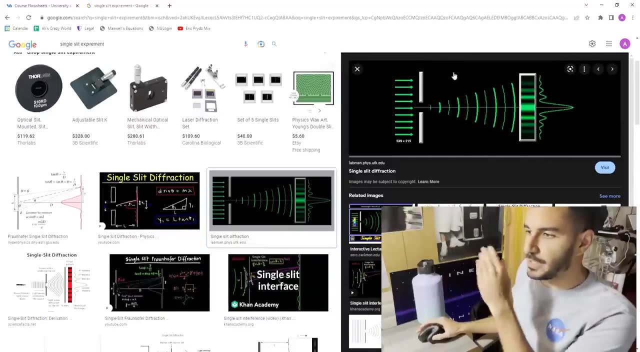 And you basically understand what it would, what, what, what putting a bunch of waves through a single slit looks like for the waves to propagate. And you'll learn what, like, this is like the near field. This is like the far field as you get farther, uh, the waves become planar and there's different ways that there's different ways to represent these mathematically, whether you're in near field, far field, and this is basically how points like this, basically how, uh, electromagnetic waves propagate. For example, if you have an antenna that propagates or laser that propagates, uh, this class is very, very, very important. Uh, you basically understand what it's like to be in the center of the sphere. So you can see that it's very important for learning 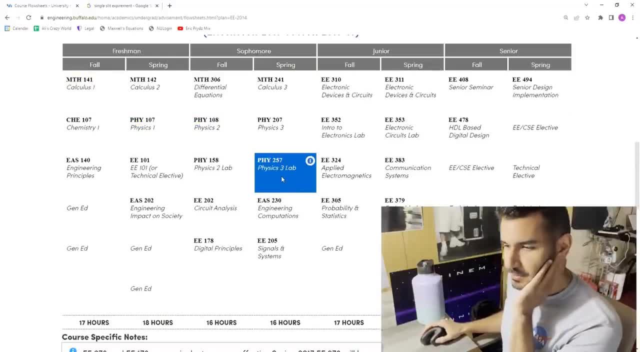 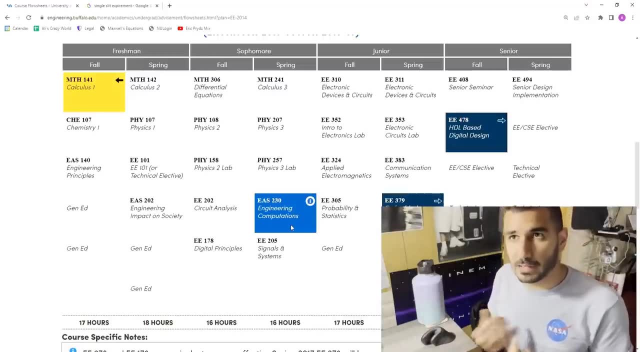 that. So physics three is very important. And then there's a lab component. Um, then there's engineering computations, and this is basically a programming class. Now, when I took it, it was MATLAB. I think later they switched it to C plus plus or Python. Uh, I think, and I really wish they kept it as MATLAB. I hope they brought it back by now to MATLAB because I think MATLAB is 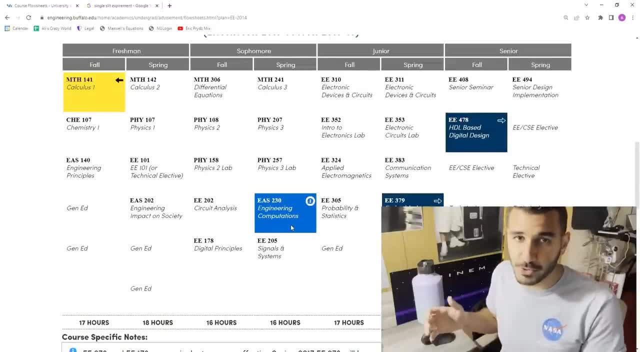 the single most important programming language for electrical engineers, for many reasons, because you can plot things very easily because there's a lot of toolboxes that are relevant to electrical engineering students. Um, and then there's a lab component. Um, and then there's a 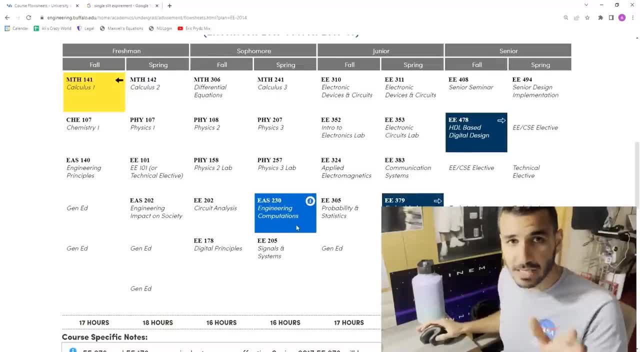 programming class. Um, so I really think that, um, MATLAB is very important. I'll probably make a separate video on the best software for electrical engineering, but this is basically 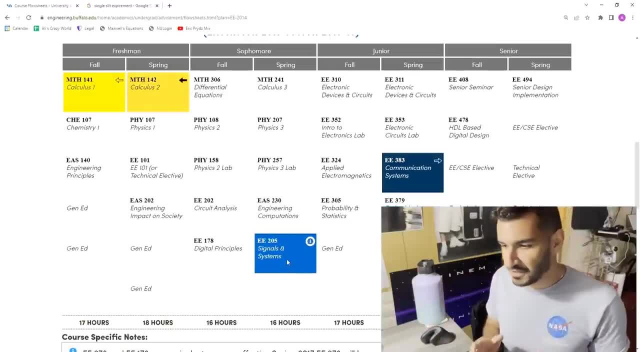 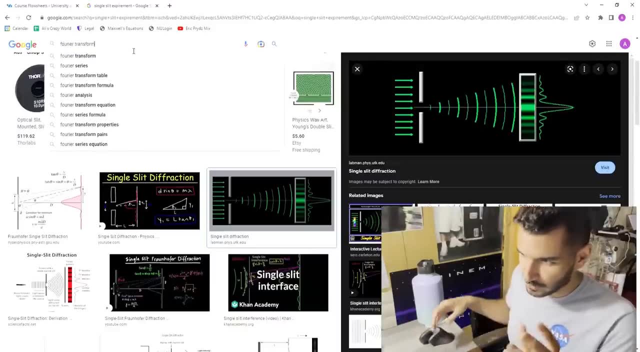 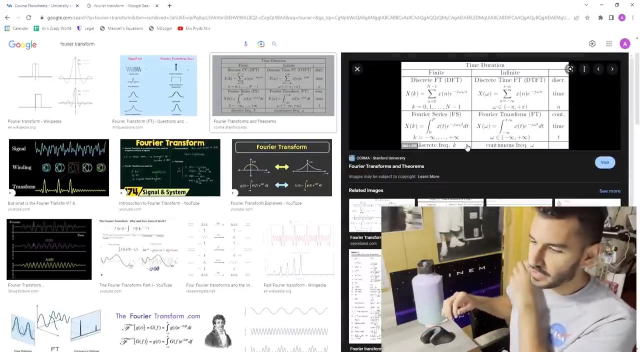 what we learned here. And then finally signals and systems and oh my God, this class is so like, let me just show you what the math looks like in signals and systems. Like let's look at Fourier transform, which is really the core. Like, look at this. Um, when you look at this as a sophomore in electrical engineering, you're like, what is going on? And when you look at this table, for example, 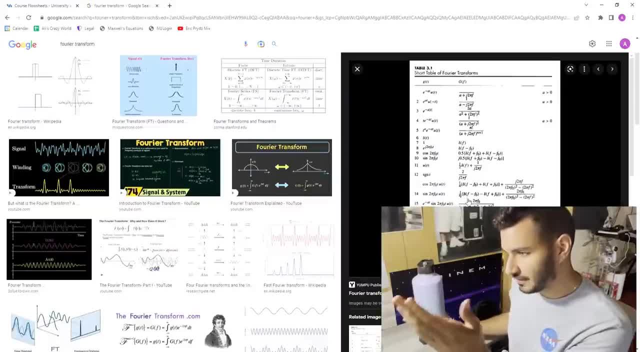 uh, of some of the, the Fourier transforms, it's kind of like a shortcut table. Um, initially it 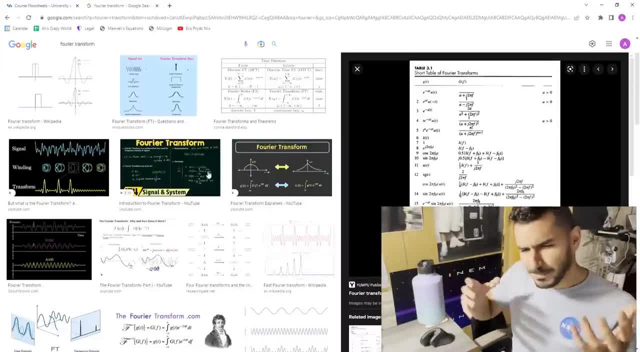 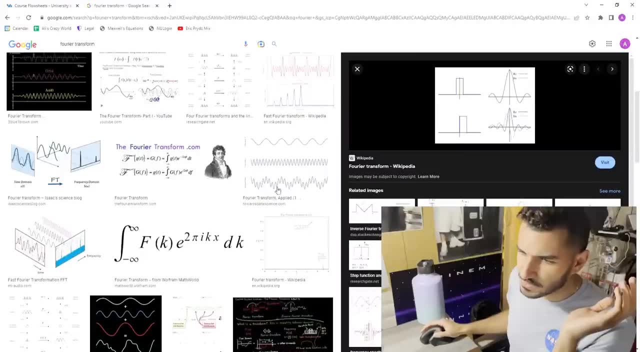 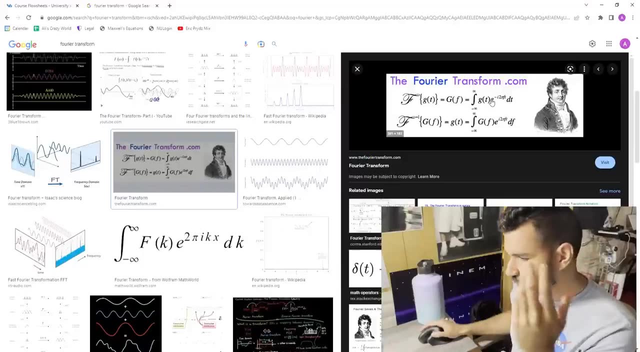 looks very intimidating and you're like, what does that even mean? What does amplitude or, or time domain or frequency domain? And what do these signals look like? And what are the properties of signals and systems? And what this guy, Joseph Fourier, he's the one to blame. Like, why did he, why did he come up with this stuff? And what is going on? This class is the math is very, 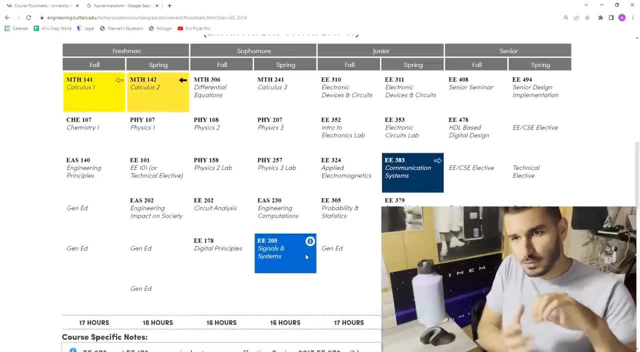 very intimidating at first. Although if you get, rid of the intimidation, the concepts really end up being very clear. 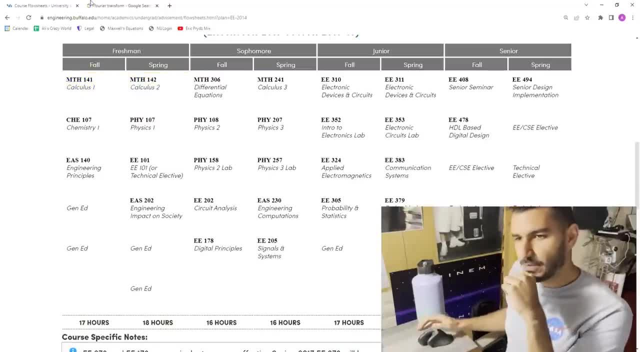 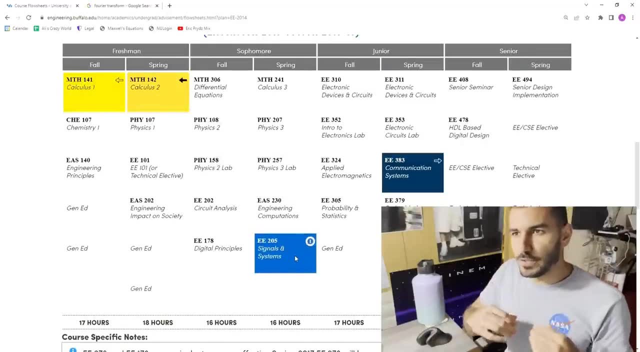 Um, because it's just that there's a lot of like transforms and there's a lot of, uh, properties of signals and systems that you have to understand. And this class is really just like a different world. So if you're someone who really struggles with like imagining things or visualizing abstract concepts, this could be really hard, but at the same time, this could help you teach, uh, help you learn those skills. This was, in my opinion, the best class, one of the best classes I've ever taken in undergrad, because it could be really, really hard, but at the same time, it could help 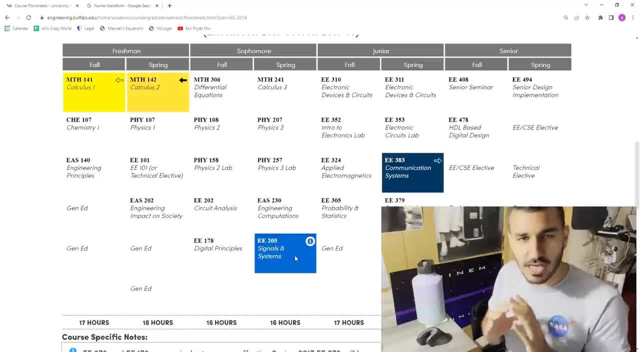 you learn those skills. So if you're someone who really struggles with like visualizing abstract concepts, this could be really, really hard, but at the same time, this could help you teach, help you learn those skills. This was, in my opinion, the best class, one of the best classes 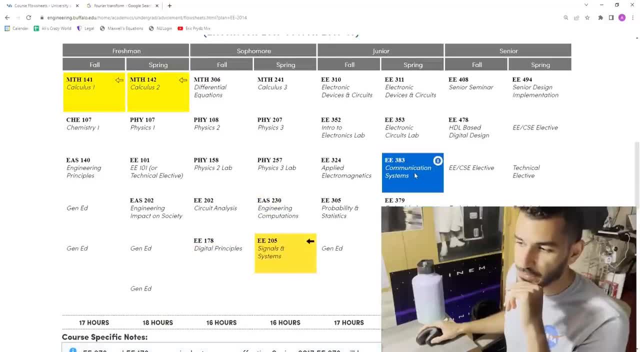 I've ever taken in undergrad, because it could help you teach, help you learn those skills. And with the follow up for that was, uh, communication systems, uh, which I ended up not only taking, I ended up teaching twice as a graduate student, and then I pursued my entire PhD in communication systems. So you could tell this, um, class traumatized me in a really good way. Um, and 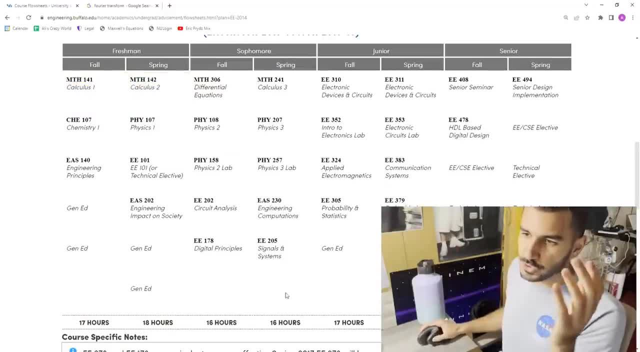 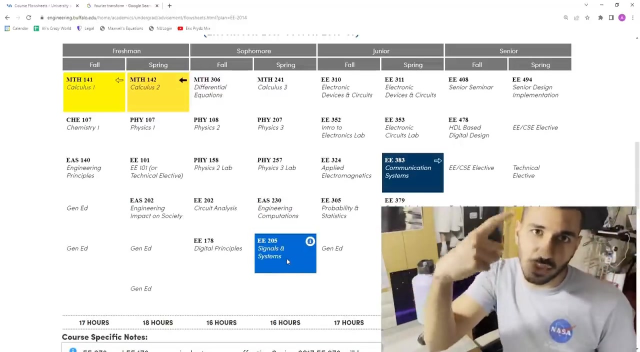 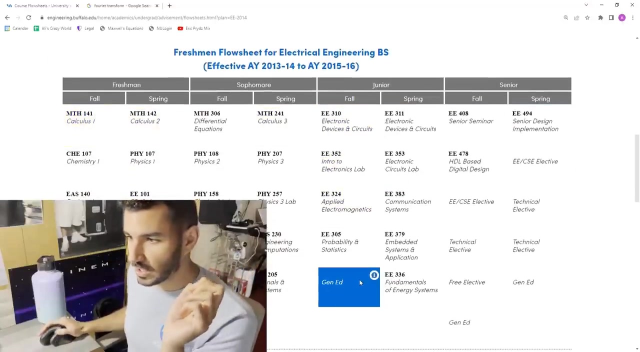 once, basically, once you take that, that's it for sophomore year. So in sophomore year, so again, freshman year, you take math, physics, chemistry, some intro courses, gen eds. Um, and then your sophomore year, you take more math, more physics, but now you're taking circuits. You're learning about binary systems and computers, and basically what builds computers. And then you're learning about how to program, and then you're learning about signals and systems and the properties of signals and systems. And signals can be anything like me talking right now to the camera or to the microphone. This is a signal like the vibrations are a signal that are being detected, processed, and then they're going to your ear as a signal as well. Um, and then the system in this case is like the channel, whether it be a microphone or the, uh, a microphone, the air or the phone that's processing stuff um and i'll make separate videos explaining these things in detail okay so now on to junior year so this is where the heavy stuff are and that is 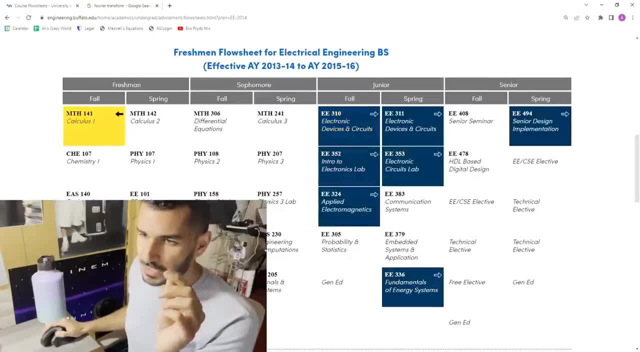 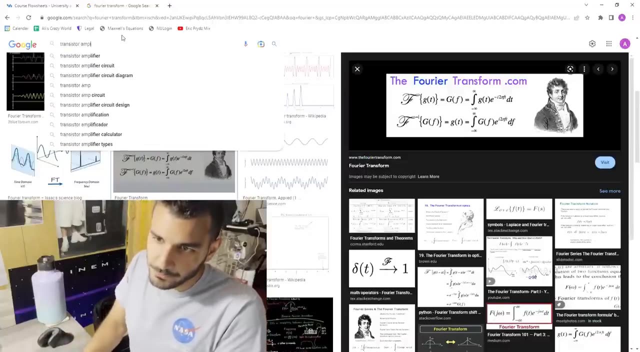 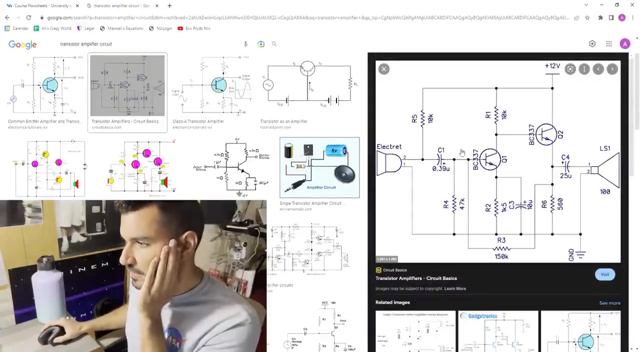 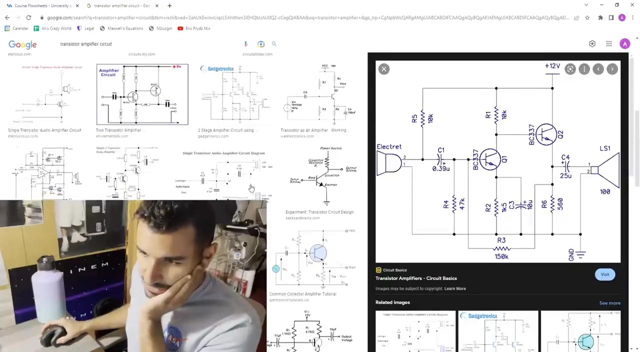 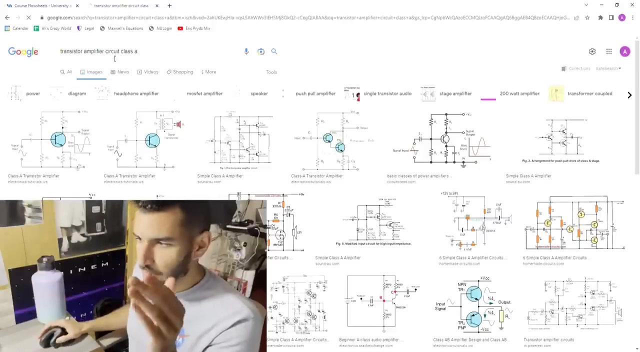 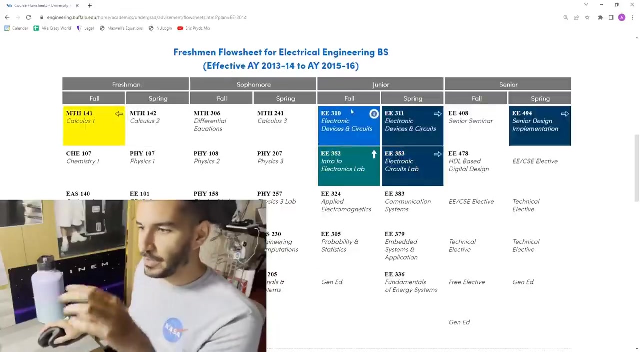 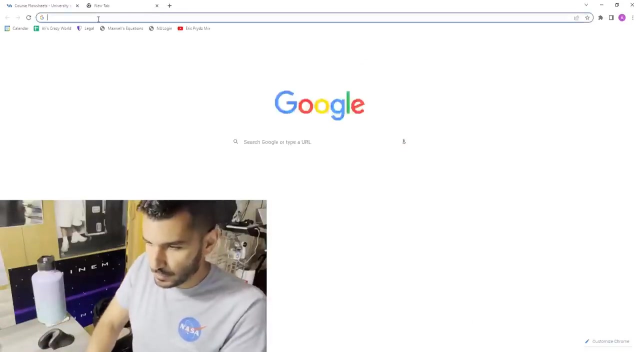 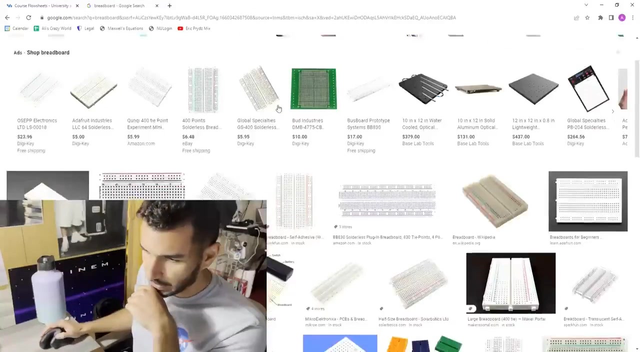 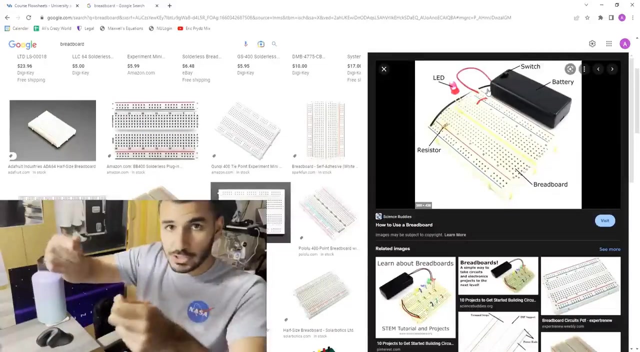 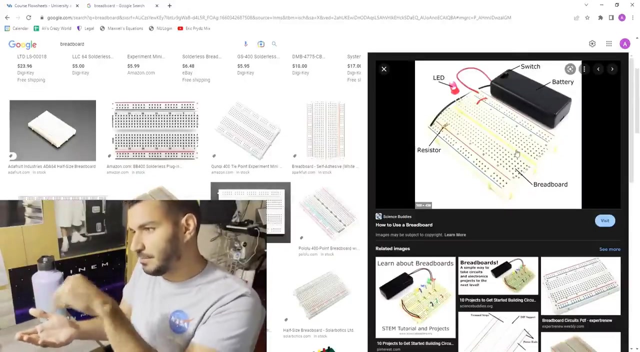 essentially your electronics so so i mentioned that circuit analysis will help you understand resistors capacitors inductors like basically electricity flowing through a wire but then once you get to the electronic circuits classes you start dealing with far more intense circuits that look like this so like a transistor amplifier circuit let's look at like a basic one um you start looking at something more intense like this where you have multiple capacitors multiple resistors and then multiple transistors right and in this case like this could be for an audio amplifier and these can get like really really uh intense based on which class um you go with they are separated by different classes of this class a class b class d depends on the application um and you you basically learn about that here in theory and then there's an intro to electronics lab so this is a very important class because you basically use breadboards breadboard and you um basically start plugging wires into things like in this case this is a um led with a resistor and a wire switch battery so this is a basic circuit and you actually get to build it hands-on using a breadboard so breadboard is again this type of i don't know thing with like a parallel metal 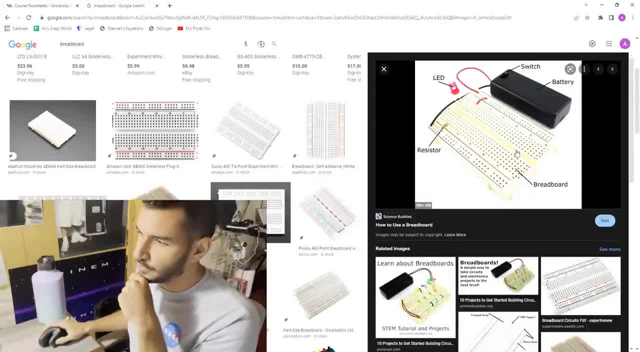 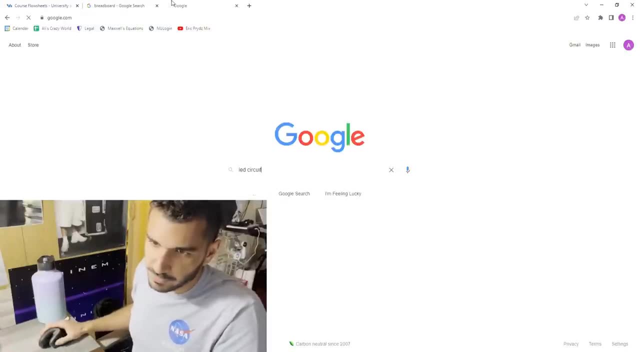 uh plates that basically makes it easier to connect things so instead of me grabbing the end of this resistor and the end of this led and kind of meshing them together i just place them in the breadboard and this line uh horizontally is connected and then this basically so this led so led circuit like a very basic led circuit this is basically what you're looking at so 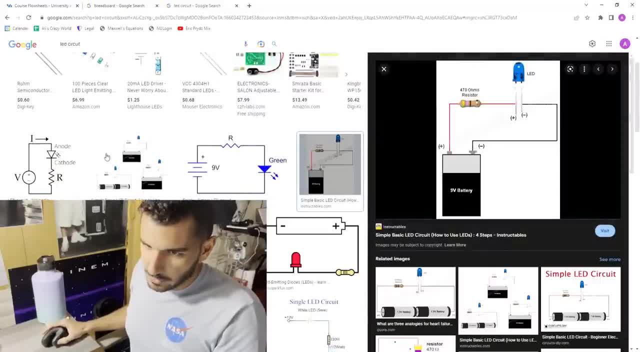 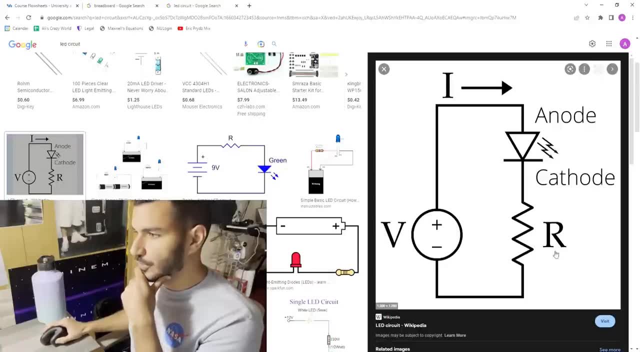 right here this guy so or like and and yeah and basic representation is what it is so you have a voltage source which current flows through because there's a resistor so there's a resistor there's a led there's a battery in this case we see there's a 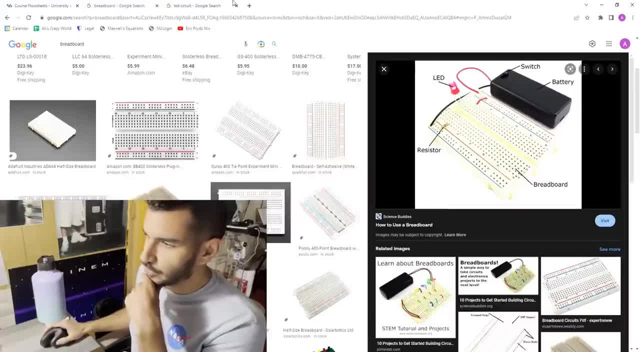 resistor there's a led there's a battery in this case there's a switch the switch you don't really see it but this switch once it's on the circuit is connected um and that's basically what these 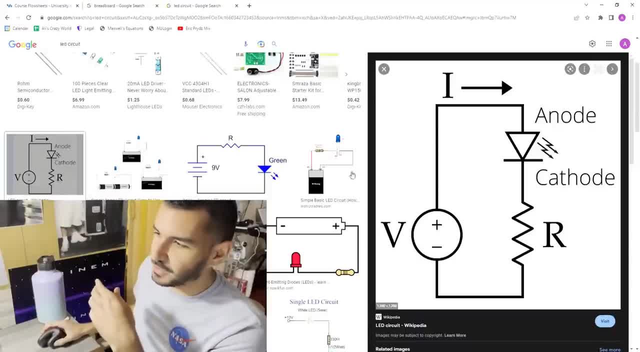 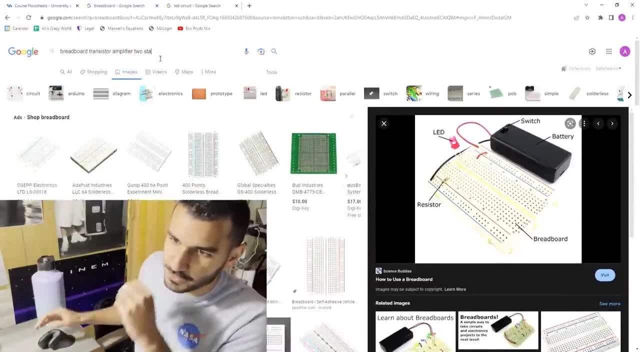 classes are obviously much more advanced like maybe this is going to be your very first project looks like this um but then like a breadboard for like a transistor amplifier two stage for example uh you start it starts looking a lot more intense right uh but it's is is very cool 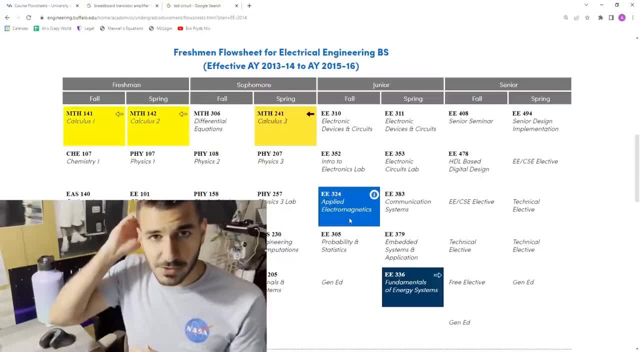 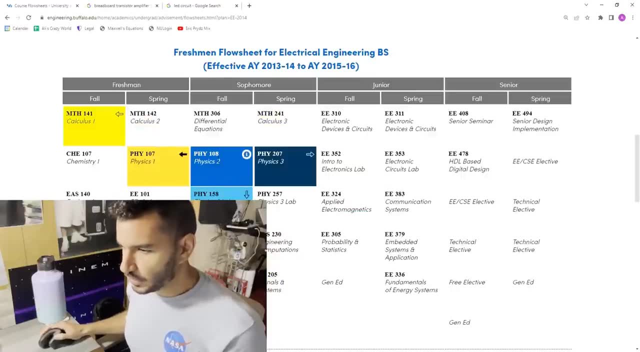 it's a really cool class um applied electromagnetics this is a continuation of physics two um i don't really know why this this is probably like a bug in the software this really should have this as a prerequisite because applied electromagnetics is like physics two on steroids 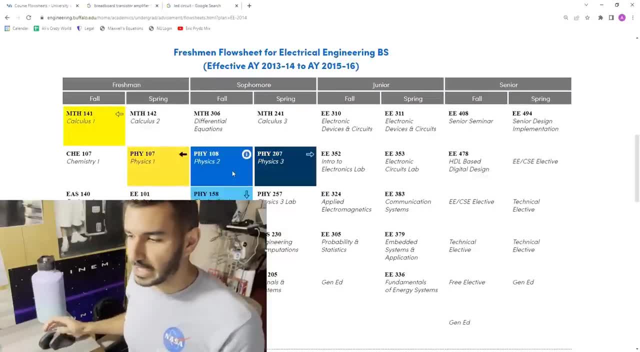 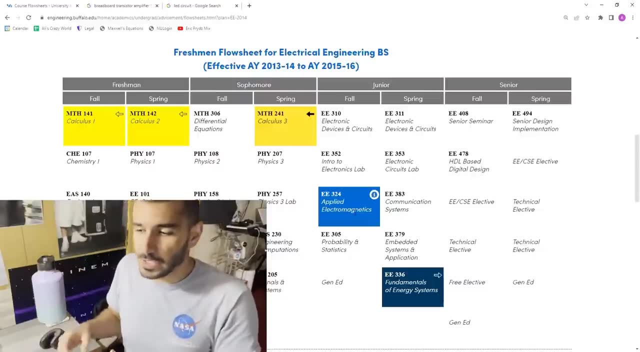 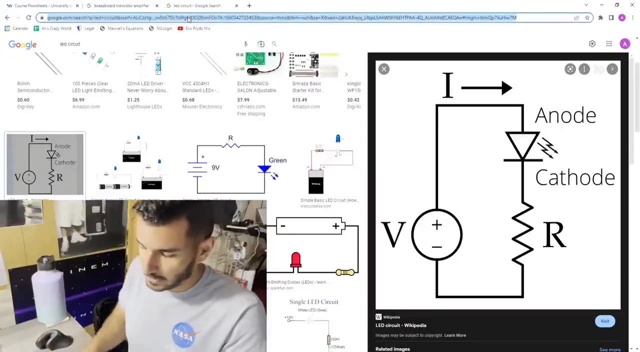 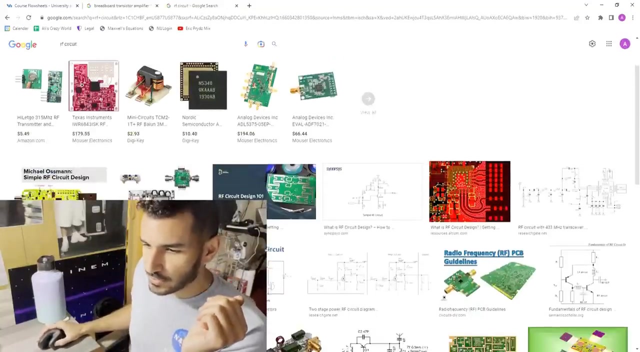 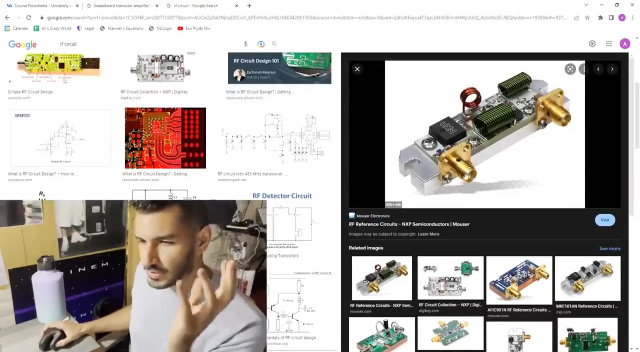 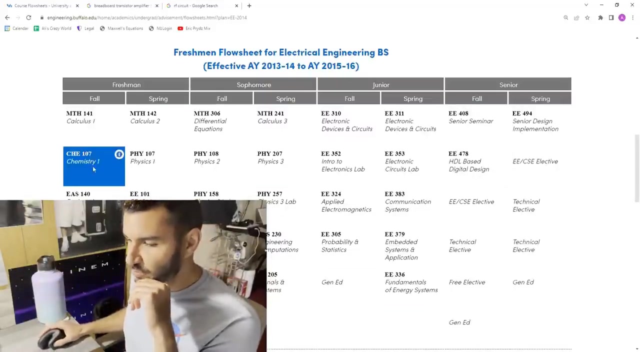 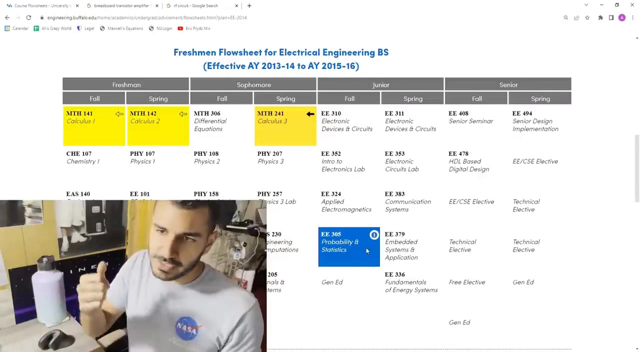 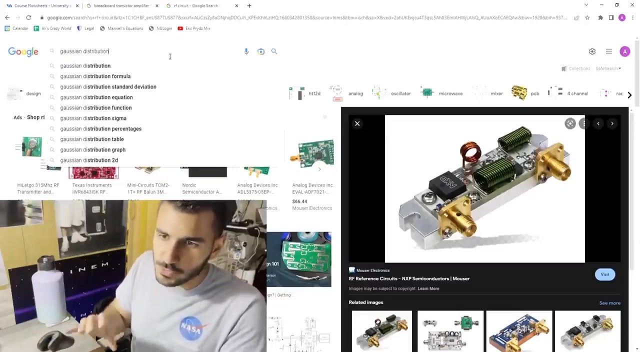 right so in physics two you learn electric and magnetic fields and in physics or in this applied electromagnetics you learn electric fields magnetic fields electromagnetic waves and how to apply them so in here you learn about antennas you learn about transmission lines you learn about rf circuits so if you don't know what like um like rf circuits look like it's basically same to these kind of circuits but with rf radio frequency so you're feeding ac current rather than dc so you do look a bit similar but now you're dealing with like coaxial uh cables and connectors and all that fancy stuff which i don't want to get into too much detail i'll make separate videos videos about these things so i don't bore you on this one with too much detail but this is a really cool class where you basically learn about electromagnetic waves antennas um rf engineering probability and statistics very important class because you learn about probability and statistics so probability theory and you start with basic like coin flips and die rolls and things like that and what are the odds that the die like like you start with these things but then you move on to more interesting things which is gaussian distributions and stochastic processes so gaussian distribution is probably the most important thing in this class to understand and that is or like a normal distribution and that is like if you take a sample 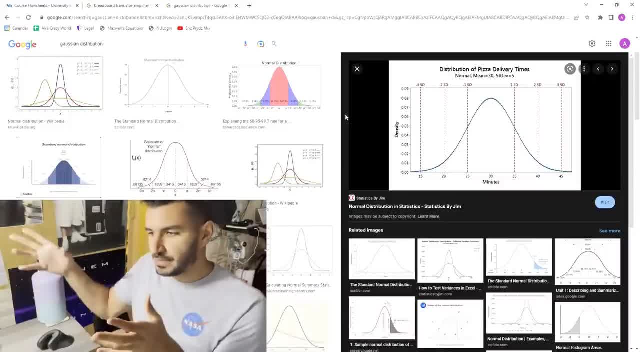 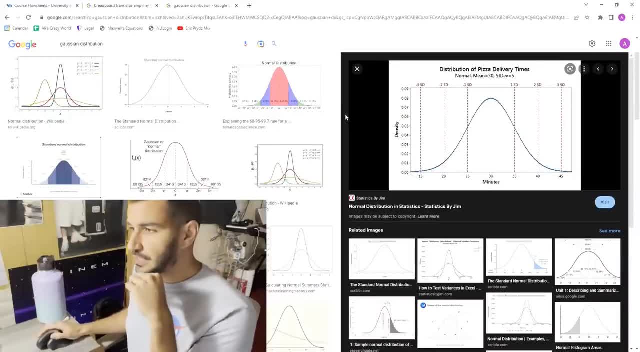 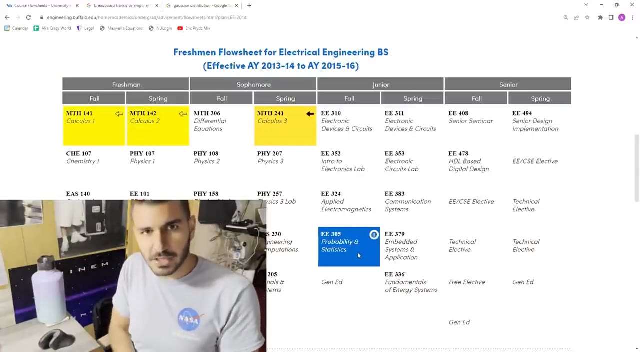 um of anything how do you represent it on this like in this case using a normal distribution curve and this basically helps you make predictions right so in this case events like like like uh when the density is higher there's more likelihood of that thing happening when when the density is lower there's less likelihood for that event to happen so this really is a class that helps you understand what is the likelihood of something taking place and and how to kind of predict um things in the future assuming you have 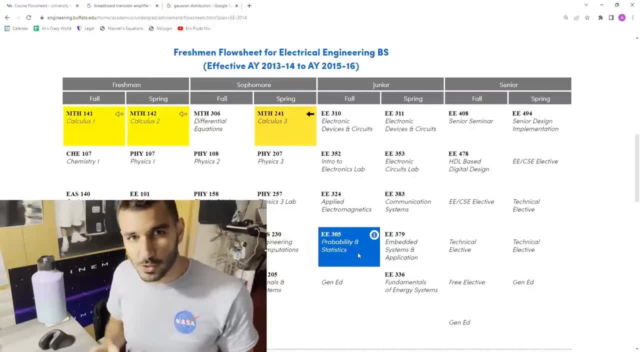 all the variables figured out now obviously in real life this does not always work because there's always like curveballs and new uh variables so there's people that try to apply this philosophy to real life and it can work to increase the odds in your favor in some areas uh but you're not 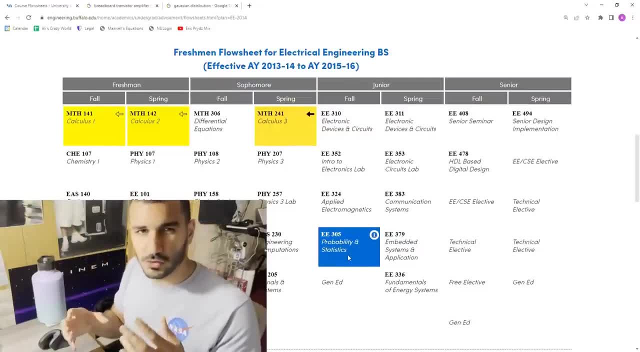 you're never never ever certain because in life there are too many variables and it's too complex to represent in simple distributions um if you're interested in that i recommend there's a book 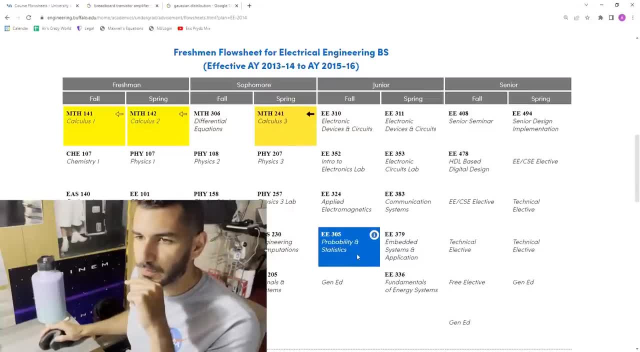 called fooled by randomness by nassim nicholas talib um it will get you a really good understanding of what's going on in the future and it's a really good book you could read uh called right here statistical consequences of fat tails and i would really recommend this if you're interested in this 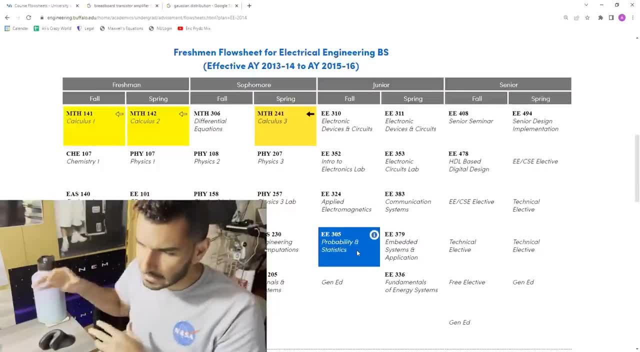 kind of um thought process of probabilities and predicting things and fat tails are like unlikely 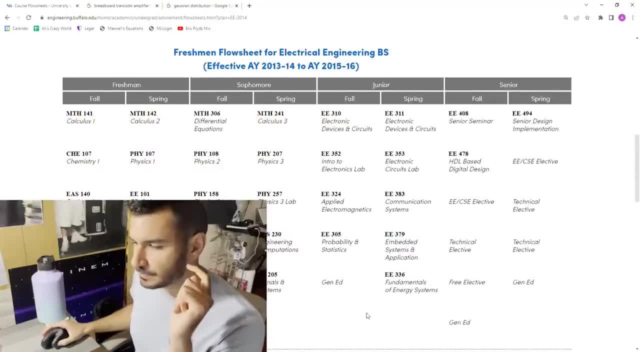 events and and catastrophic events and things of that nature um so yeah you should probably look at that and that basically takes care of the fall and then in the spring you take the 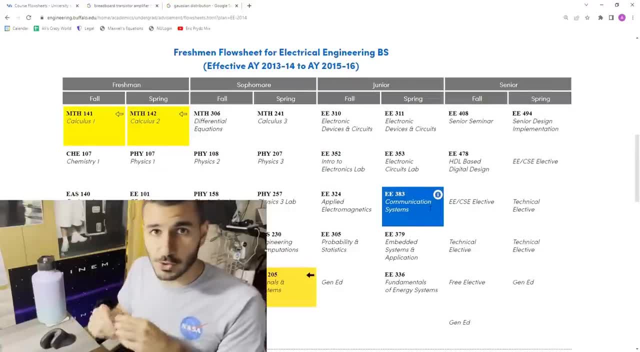 continuation of the circuit class the electronics the lab and then here you learn about communication some communication systems you learn about basic transmitters channels receivers 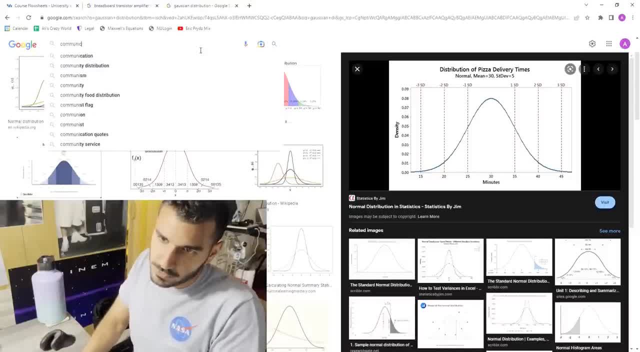 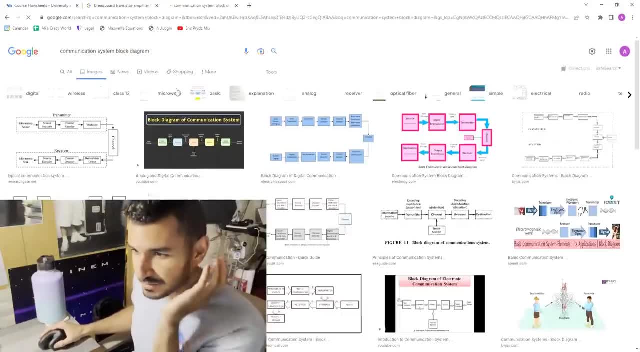 so basic communication system system block diagram is what it would look like um well we don't really need an explanation we just need the block diagram because i'll provide the explanation 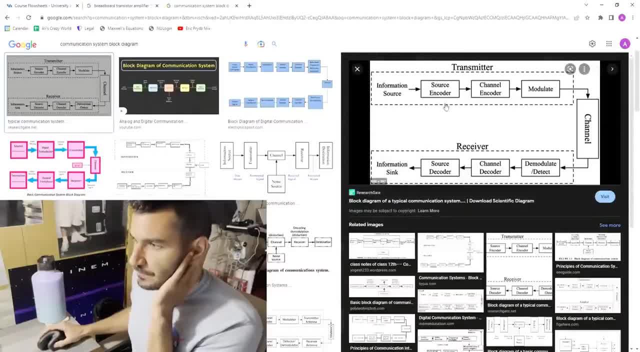 so in this case if you have your information uh like in this case your ones and zeros uh the encoder source encoder i think just basically gets rid of any redundancy um the channel encode well 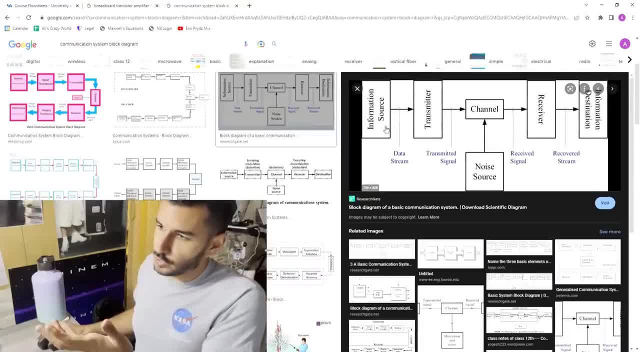 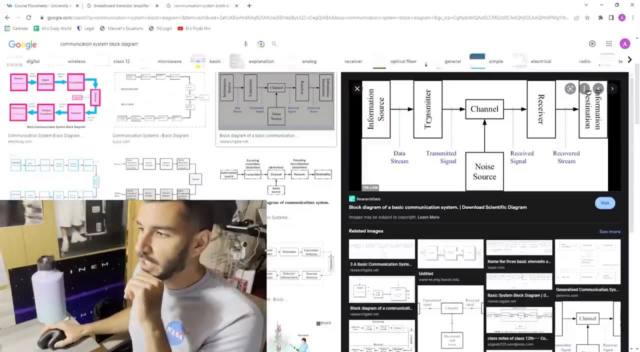 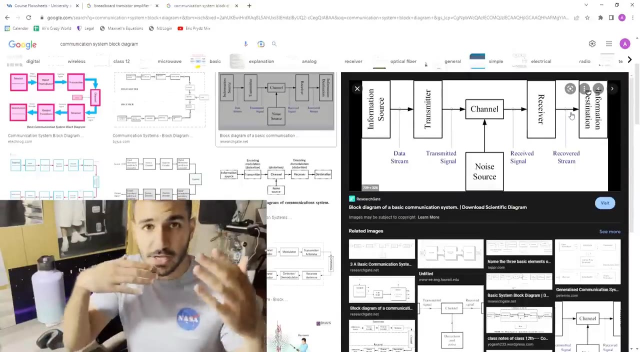 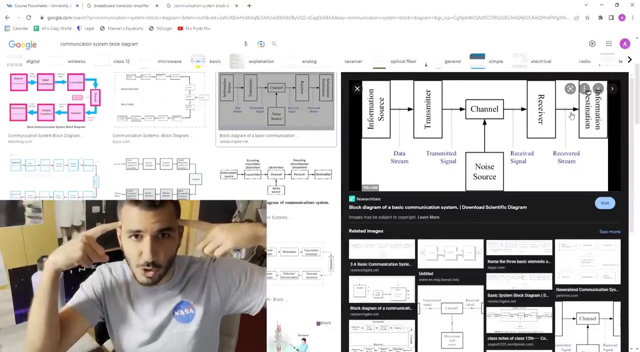 let me go over here there's a much simpler one so in this case you have information source ones and zeros transmitter something that takes those ones and zeros and sends them in the air so in this case like a radio channel which in this case let's say it's air because the air has molecules and other signals there will be noise and then your signal is received by a receiver in this case also has a radio um and then the information is decoded so you get your ones and zeros back so in this case what this is a communication system so my mouth is my brain is the information source my brain is coming up with ideas and words and you can think of those as the ones and zeros and 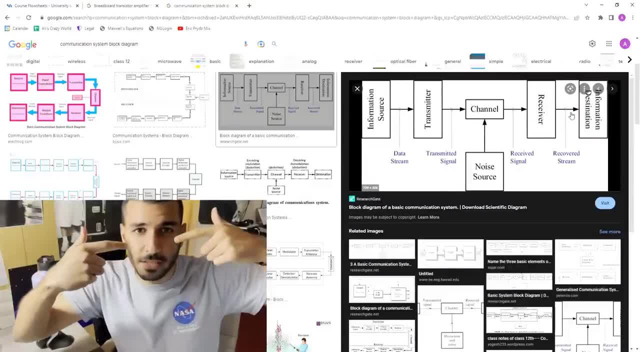 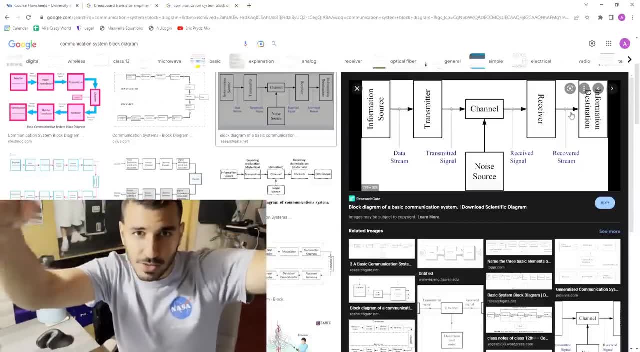 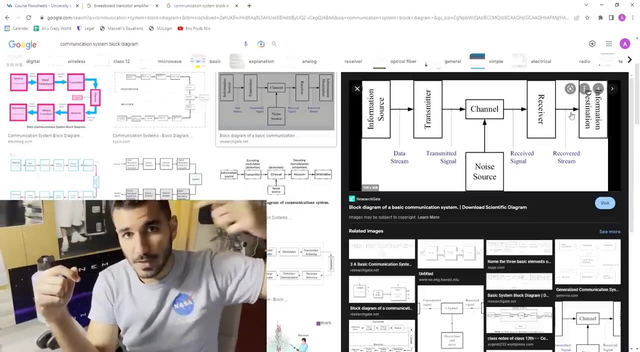 then i'm taking those and i'm modulating them i'm equipping them on my mouth and i'm making vibrations with my mouth as a transmitter so my mouth is propagating those signals and then um the channel is the air right so the my words or my signals are traveling through the air and then your ears are the receiver in this case so your ear would be this receiver and then basically your 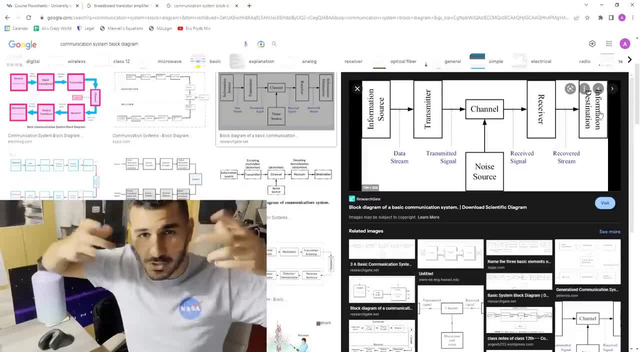 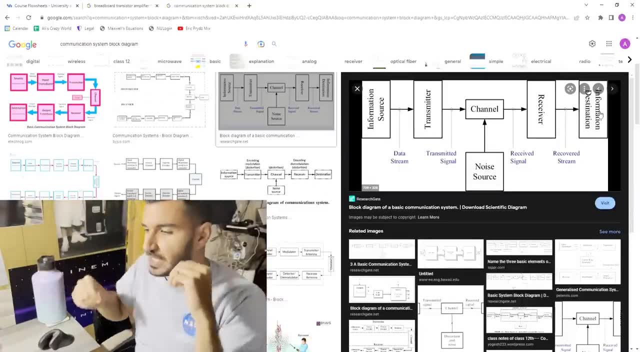 so your brain will take those sound weird sounds that i'm making and interpret them because you understand english hopefully if you made it this far in the video and um you're you'll be able to understand the meaning okay and that's basically the foundation of communication systems it's 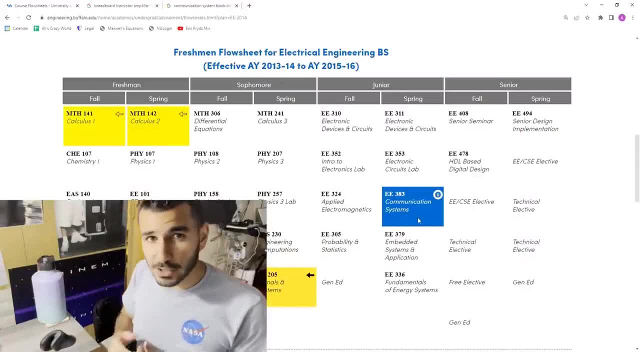 awesome again i love comms uh my work is on satellite communications so satellites talking to each other i'm trying to make satellite communications faster um so yeah awesome awesome 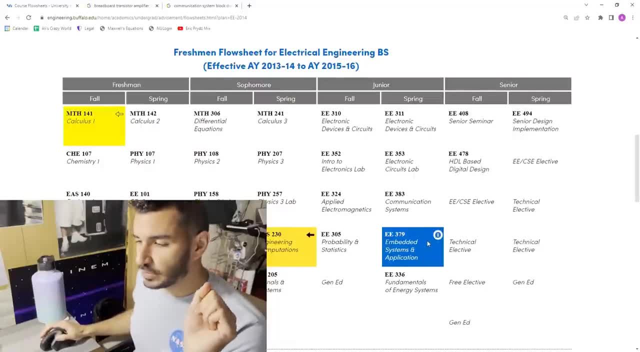 class embedded systems is a really fun class because you get to do things that are hands-on 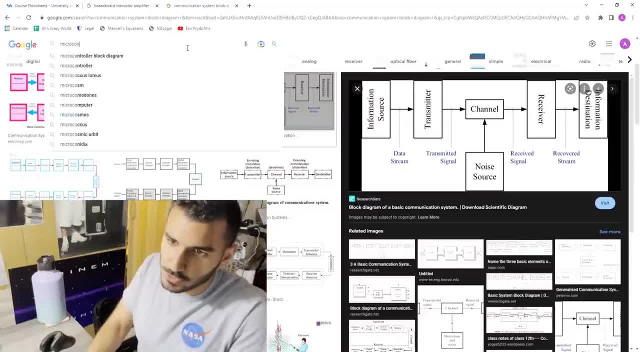 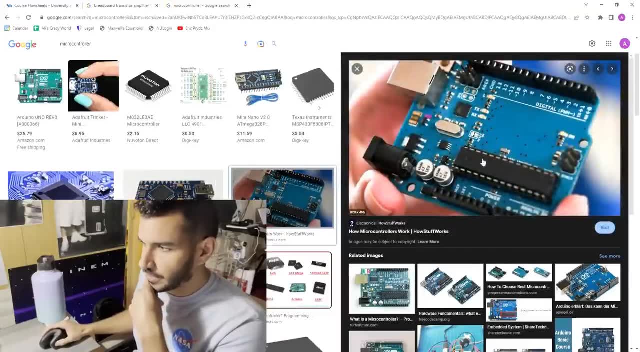 so here you learn about microcontrollers so here you learn about microcontrollers so here you learn like a microcontroller it's basically like a mini computer that you can work with and like for example there's an arduino microcontroller as you can see there's like a little chip here and there's connectors uh and there's other stuff going on and there's like power supply there's like another i think there's another also for power and you can basically uh use this to build 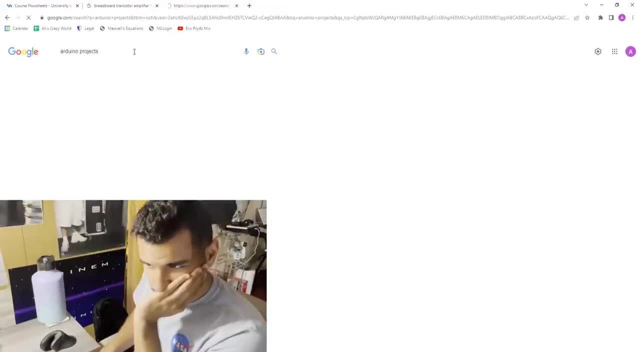 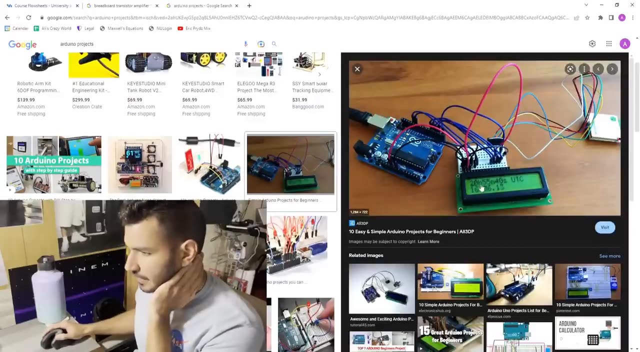 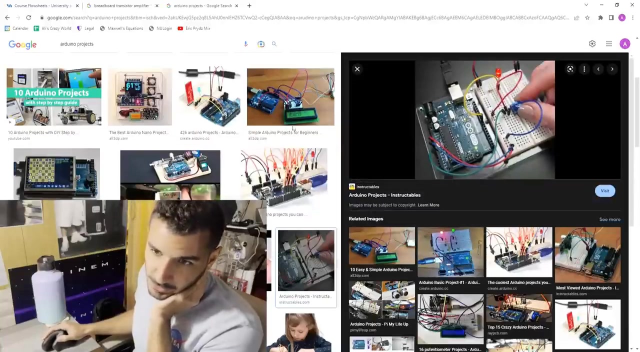 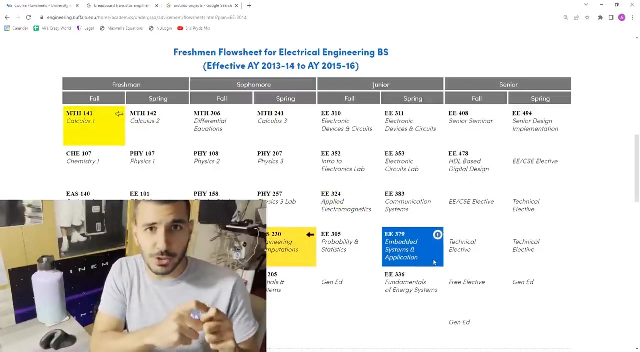 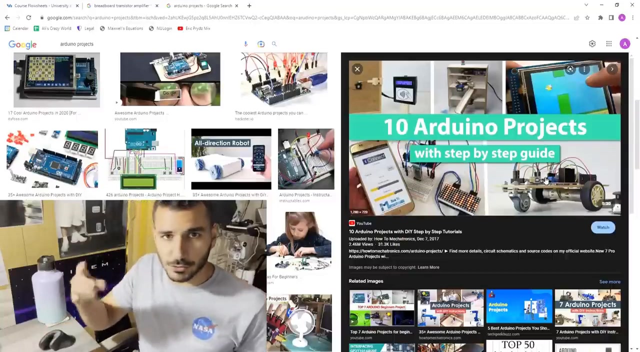 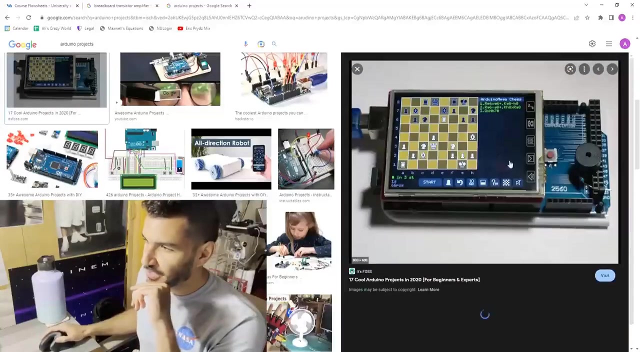 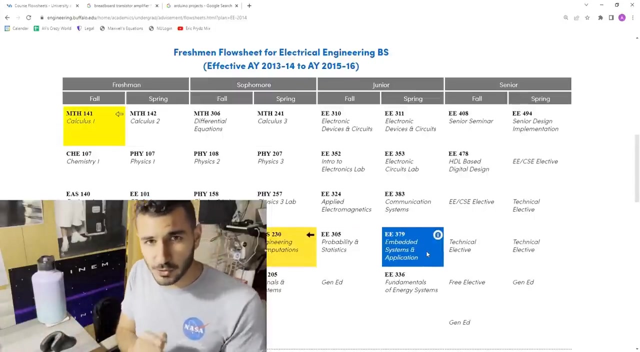 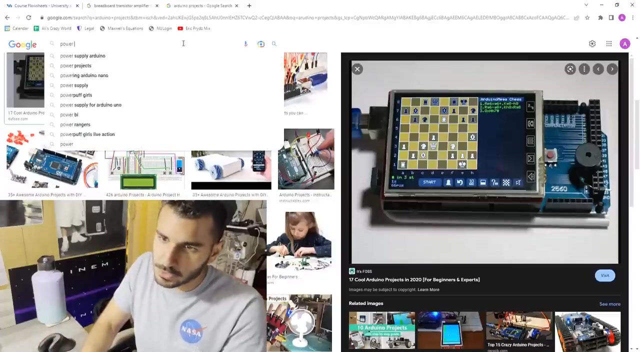 projects so like arduino projects so in this case you have like a lcd screen that's demonstrating uh something i think it's telling time yeah so this is actually a clock uh it's pretty cool um or like i don't know like this circuit is doing something or you could use it to like build like moving vehicles or whatnot so you're basically in this class learning about um small computers that serve specific application and basically how to program those small computers to do what you want right and you'll learn about sensors and actuators like for example in order for this car this this computer is going to have to tell the wheels to turn right it's going to have to tell like an led in this case or lcd to blink right um or in this case this you can you can play chess with it which is awesome i love chess and that's basically this class is very cool and especially if you're into programming but you still want to pursue electrical engineering this is very this is the right area to be in also if you're into computer engineering this is the right area to be in because computers the microcontrollers are small computers essentially um and this is what you would be learning and then finally there's the fundamentals of energy systems and this is where you learn about energy systems and power grids so like power grid and how what 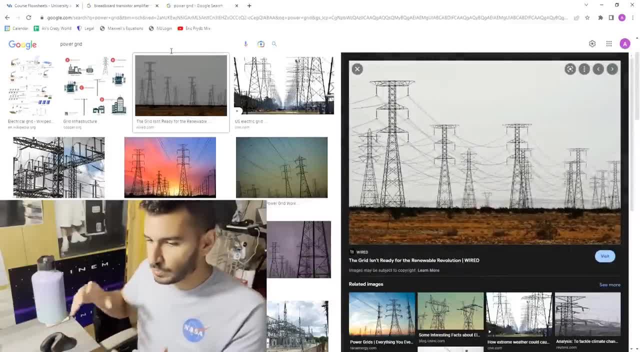 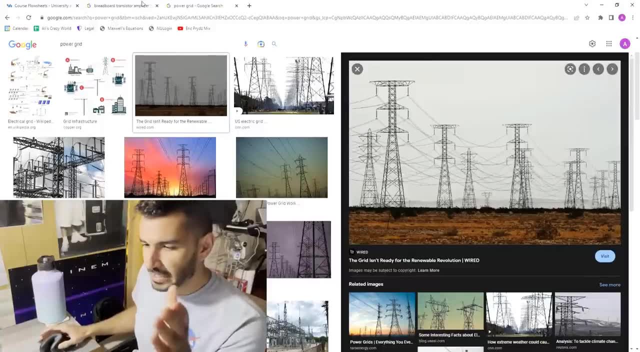 these guys how these guys operate and like three phase energy and what that means and how the energy is distributed and the efficiency of how efficient are you um at being able to carry power from point a to point b and all the economics involved in them um so if you really like this uh power 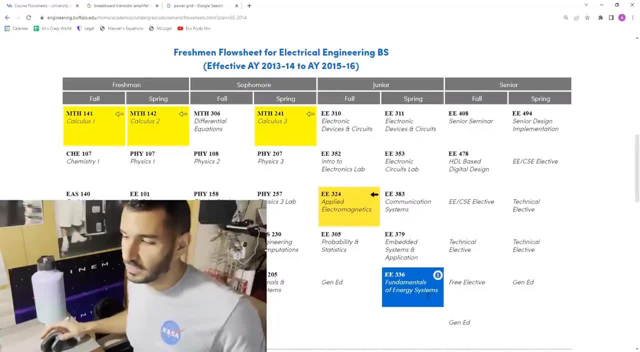 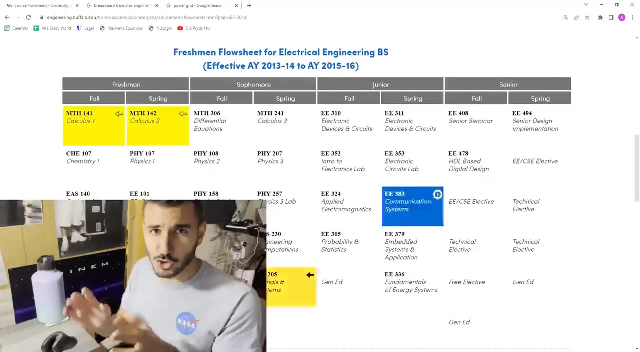 systems or energy systems if you really like large numbers like uh watts kilowatts megawatts gigawatts uh this is the class for you because you end up understanding how these massive amounts of energy are generated and then transferred um and so forth and that basically covers junior year engineering again is kind of the most intense because you learn a lot 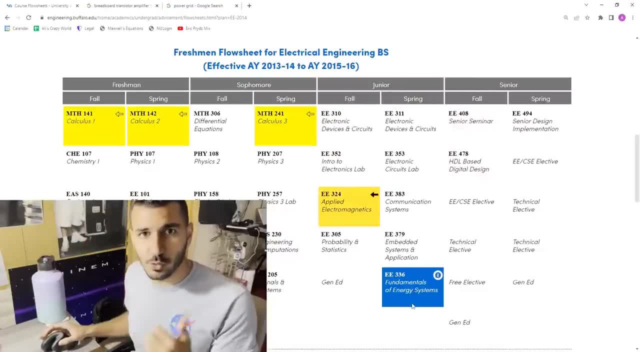 hopefully by the end of junior year you have figured out which class you like the most and which one you want to specialize in such that all these electives will be hopefully in like one or two areas that you really liked for me the class i like the most were applied electromagnetics and 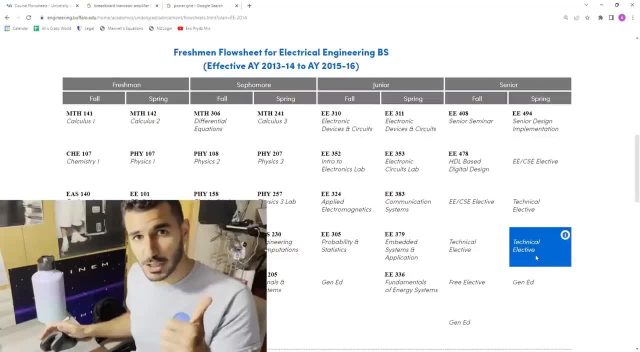 systems so for my electives i ended up taking more rf communications antennas microwaves as well as digital communications i think radars bio communications things like that but then you do have a senior seminar which i think there's like a professor that gives you advice about what to do 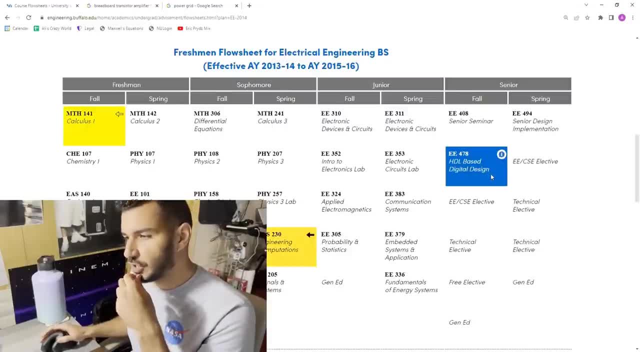 um in the real world um hdl based digital design uh this is a very cool class because in digital principles do you remember those ones and zeros i showed you in hdl you get to program them directly 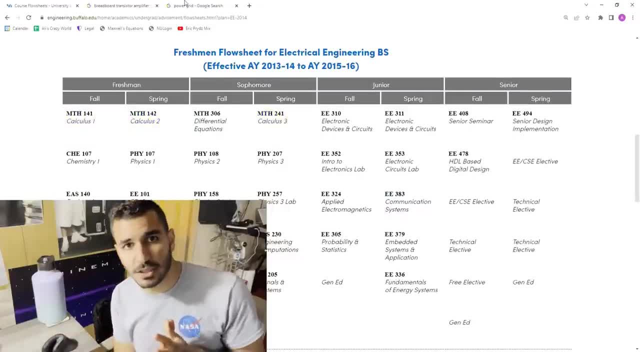 so like in normal programming like python or c plus plus uh you write code that compiles into assembly language which then compiles into ones and zeros and then these ones and zeros tell the transistors what to do uh an hdl based uh program and hdl stands for hardware descriptive language 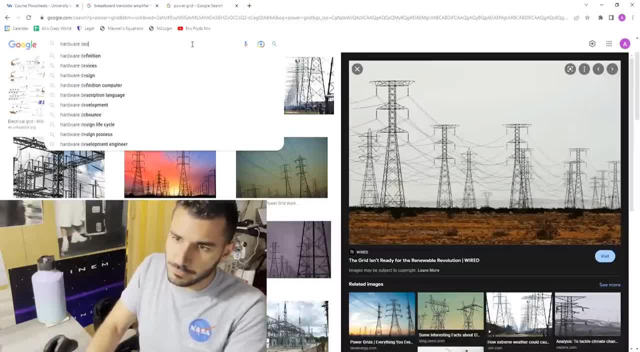 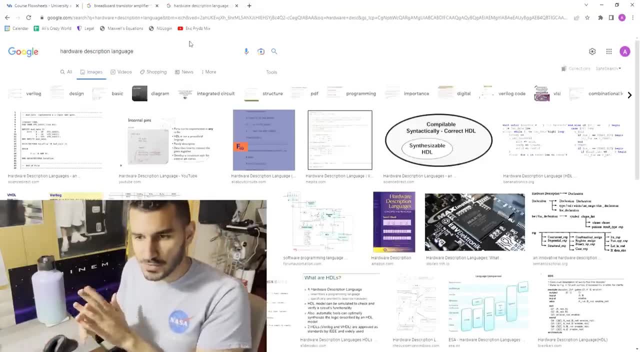 i think so hardware descriptive language yeah and in this case you're bypassing this um compilation of hardware and you're going straight to the hardware so you're literally building these things 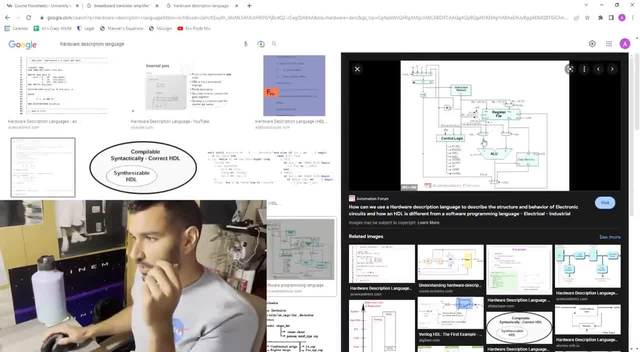 in code so you're building alus you're building logic gates uh you're you're directly calling on registers and memory um so this is a really cool class again if you really enjoy computer 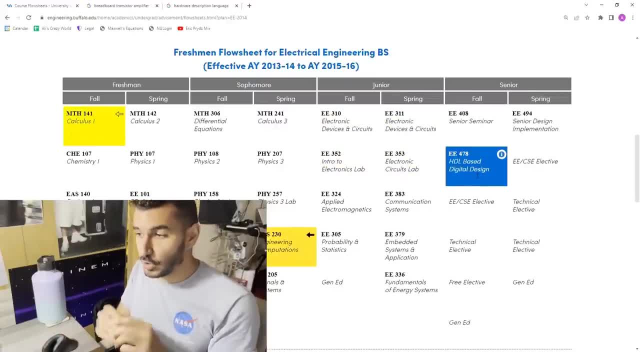 engineering concepts or this uh digital principles or digital circuits in general these are these are this is the foundation for digital circuits um but it's cool because you 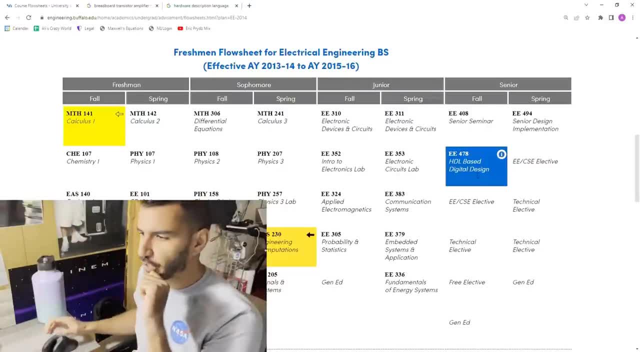 basically program them rather than like draw them in circuits um and then finally in the spring you have your senior design and then you have some more electives and senior design i think you get 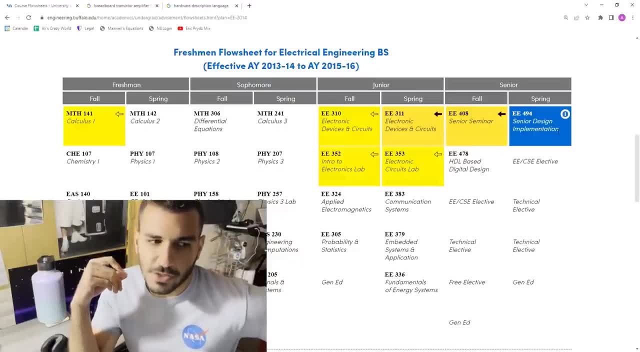 together with a bunch of people and you build something and then you present it and then they clap for you and then they hand you your degree and then you have a bachelor's in electrical 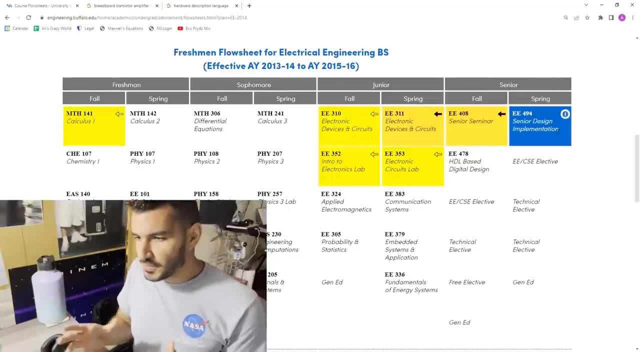 engineering um so this pretty much covers it in a nutshell i know i was speaking really fast 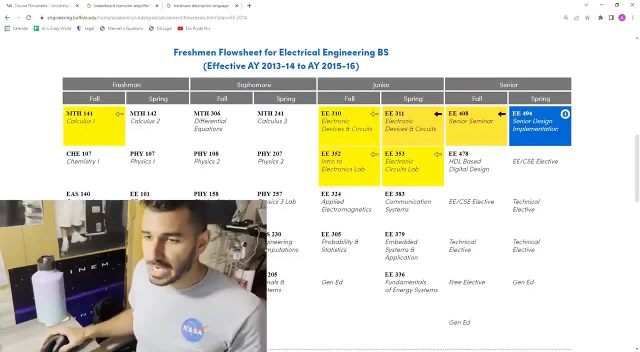 um one important note i want to mention as you're taking these classes like freshman sophomore 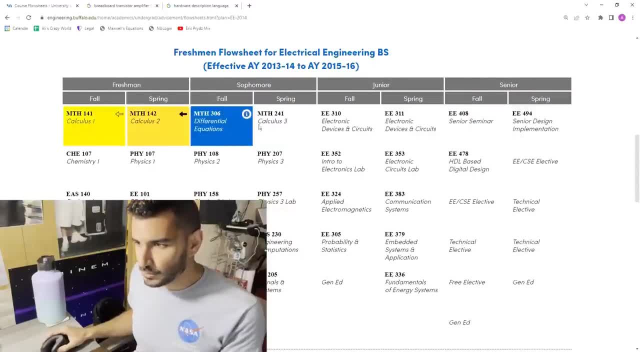 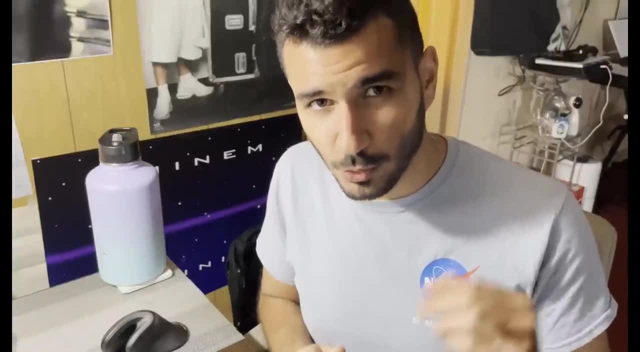 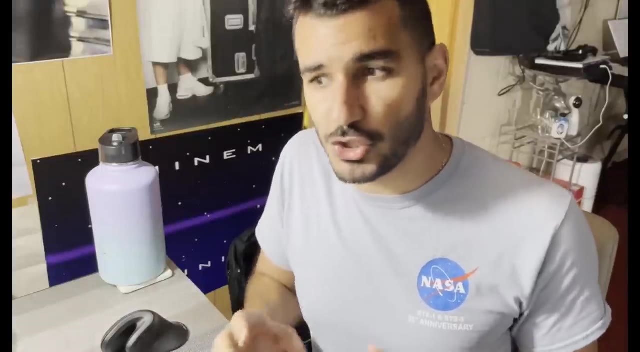 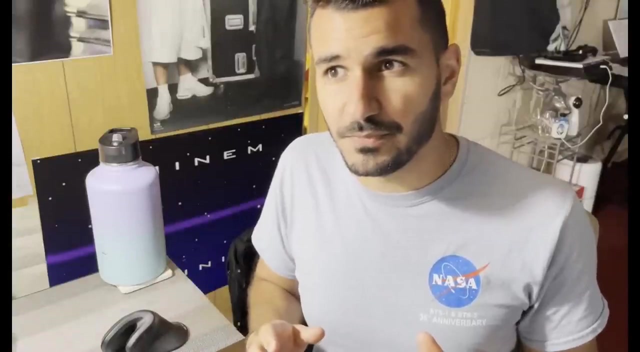 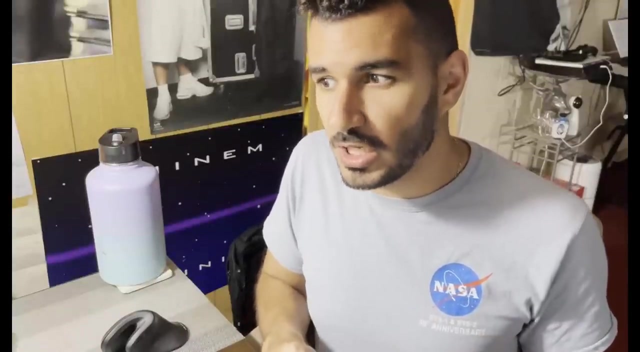 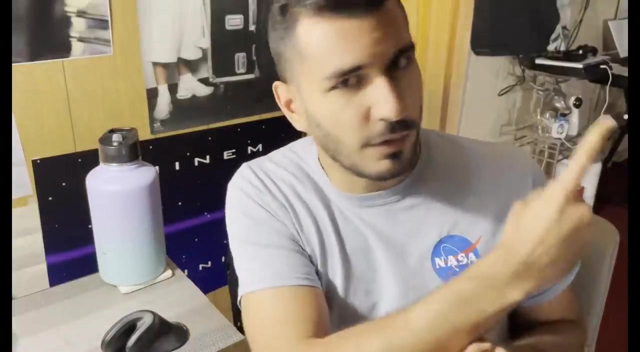 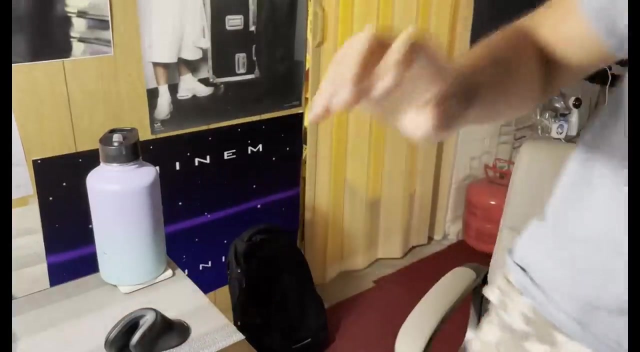 junior senior you want to make sure that in these summers between them you're doing internships right internships are extremely important if you have not done one before don't panic it's not the end of the world you can still get one or you can still do some sort of project that can represent an internship or something like that but in electrical engineering classes are important because that's where you're going to learn the basics but more important than classes is getting um real world experience and internships and i've done many electrical engineering internships and i loved all of them and they taught me so much and i'm going to put a link in the description for electrical engineering internships and how you can learn from them and it might even show up over here so you should check that out if you haven't already peace love 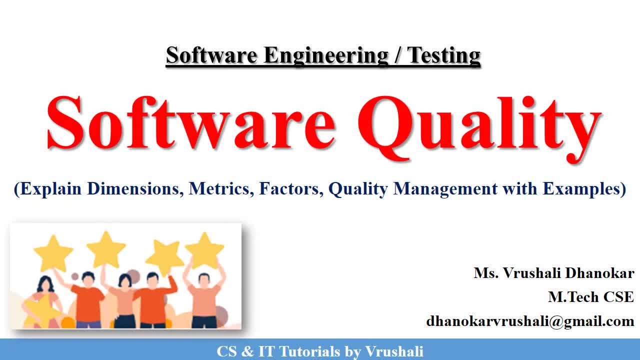 Hello everyone, this is Rishali. In previous session we discussed about all types of testing. with example, I have mentioned complete software engineering. subject playlist link in below description box. Now in today's session we will discuss the next important topic that. 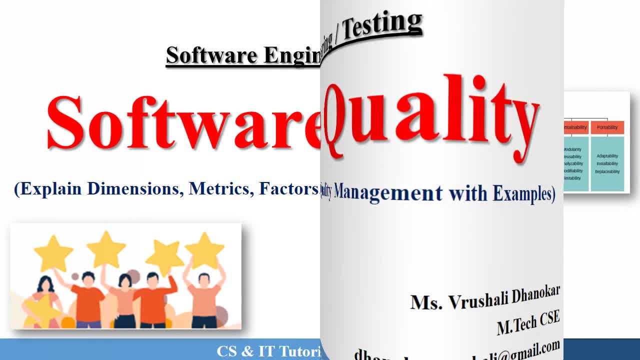 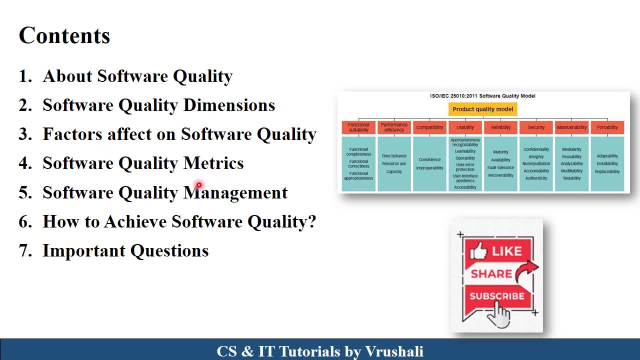 is software quality. Let's start the session. In this session we will discuss about software quality. there are dimensions, factors, matrix, then quality management and how to achieve software quality. At the end we will discuss some important questions that have asked in.